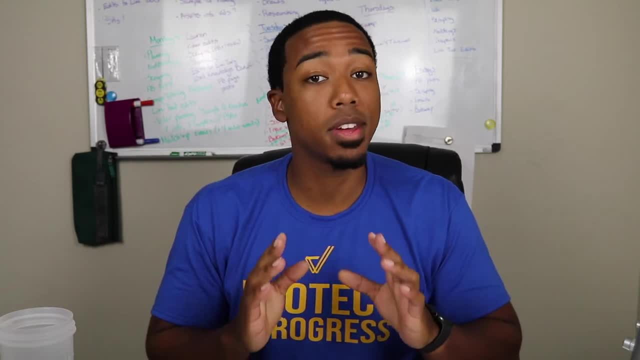 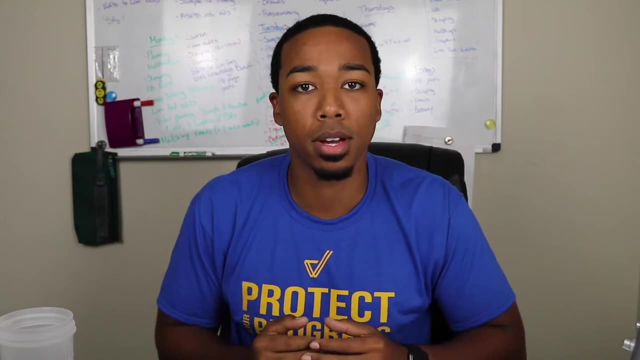 first I'm going to say that one more time. Don't go through the information, Just go straight to the question statement. If it only has one sentence in the question, great. If you have three or more sentences there, You know a word problem? Well, just go straight to the question. Because here's the thing: When 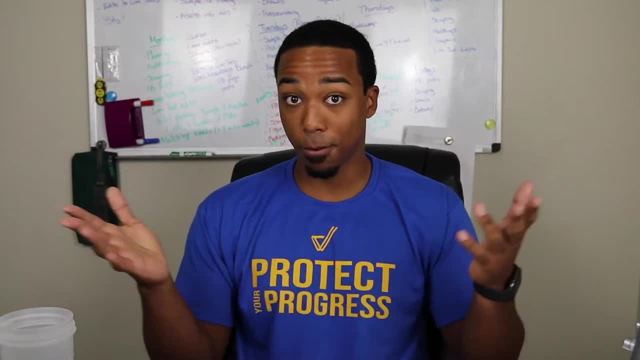 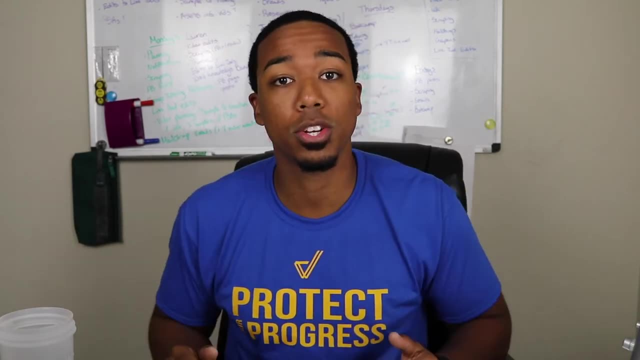 we want information. do we end up getting the information all at once or do we pose a question first? So think about how you search for information online. You have to put in the actual question in Google before you can actually get the information that you want, And that's because you. 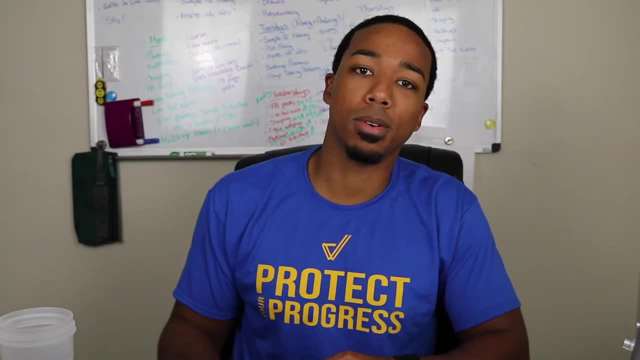 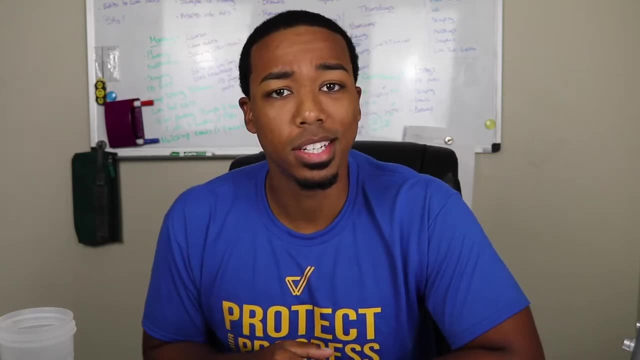 know what you're looking for. right, And now let's think about another example. Let's go ahead and think about, well, the whole analogy of you don't get in your car and drive unless you know where you're going- I mean, that's a pretty self-explanatory statement right Now, let's go ahead and apply. 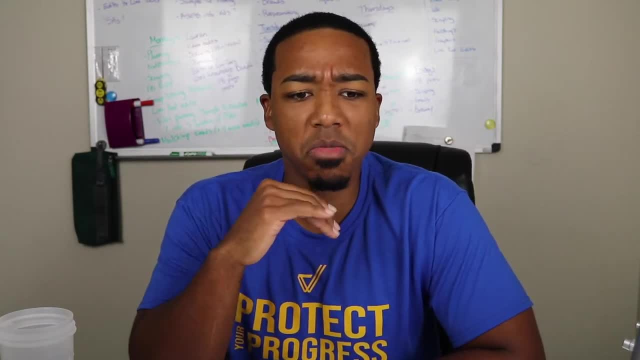 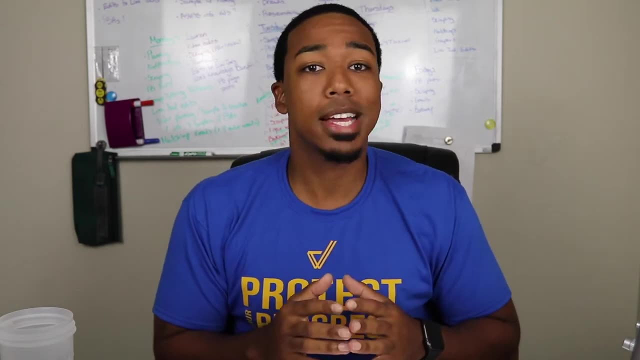 that to word problems. So let's go ahead and say: you know the average person- and this is a true statement, because I've been doing this for about 11 years now and I've seen this way too common Most people. what they do when they read a word problem is they get fixated on the numbers first. 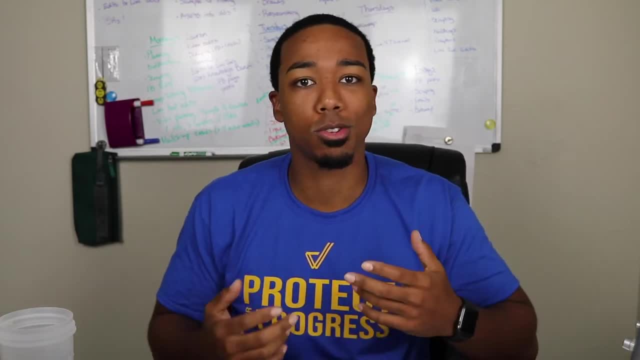 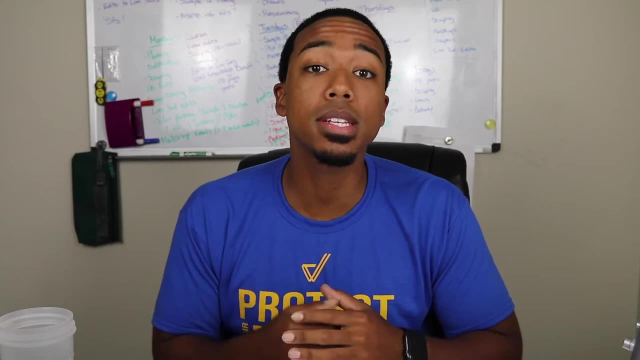 You know, they go straight to the numbers and they start calculating together with those numbers and then just hope for the best. Maybe single Hail Mary here and there, right, But the thing is that's not going to get you anywhere at all. And the reason, again, is because 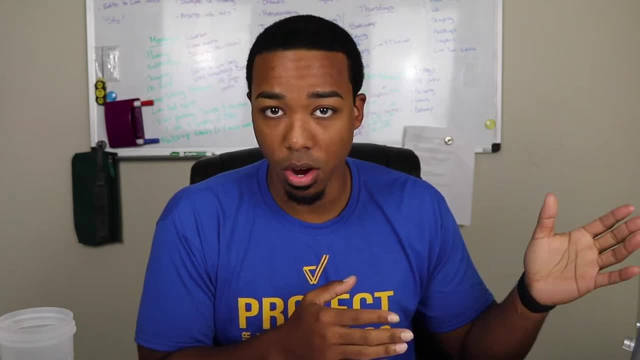 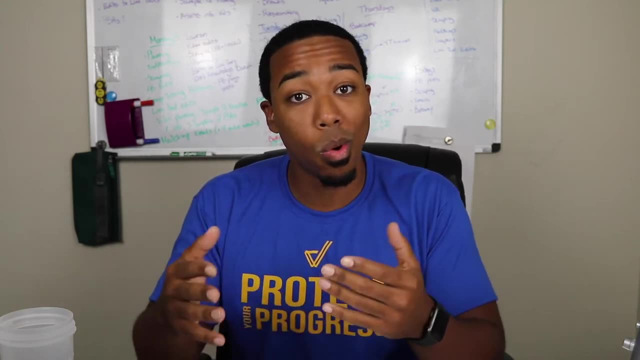 before you get in your car. typically, you know where you're going to go, You know what the destination is, You know where you're going, And so when you start a word problem, you need to understand what the question is, what you're answering, what you're trying to figure out. All. 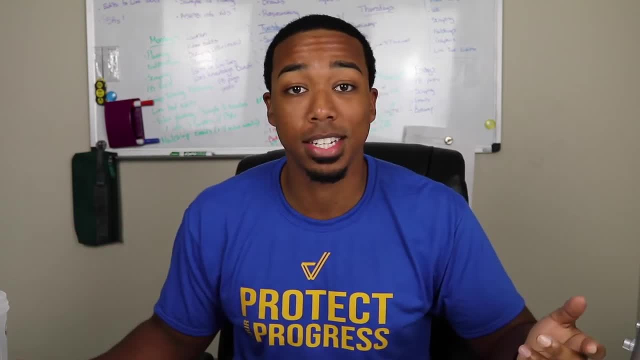 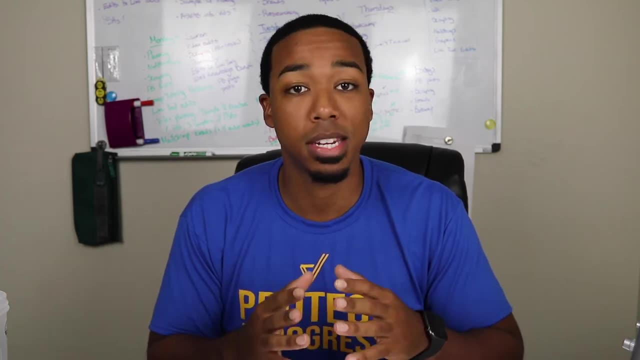 of the extra information. it's just extra information, It really is, until you know what its purpose is. So the numbers don't get fixated on those, Just get fixated on what the numbers mean at first. But before you even do that, again, you need to know where you're going. So let's go. 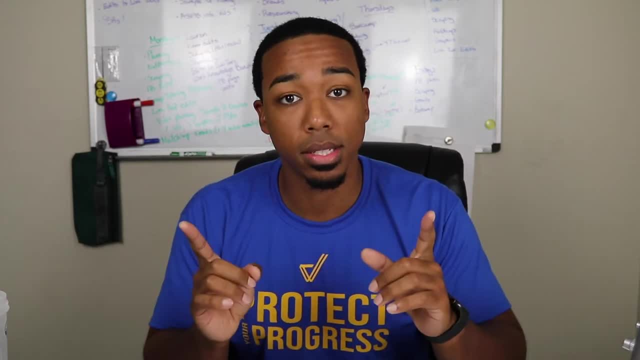 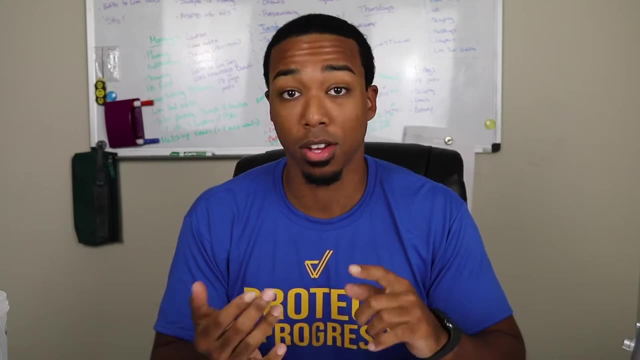 through the methodology You get in your car, but before you do that, you know where you're going. Great. Now, when you get in your car, you can't just speed off Because, remember, if you have a car, you know good and well that the car needs to warm up first, The oil needs to get hot And two. 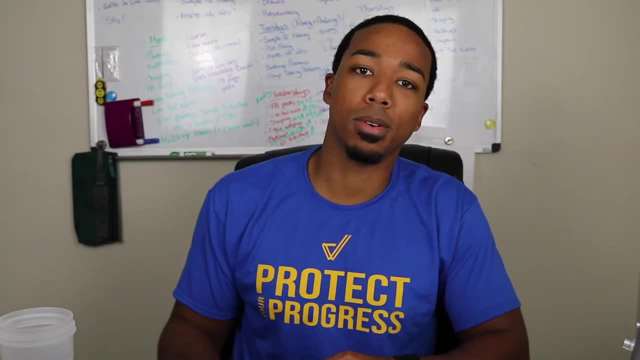 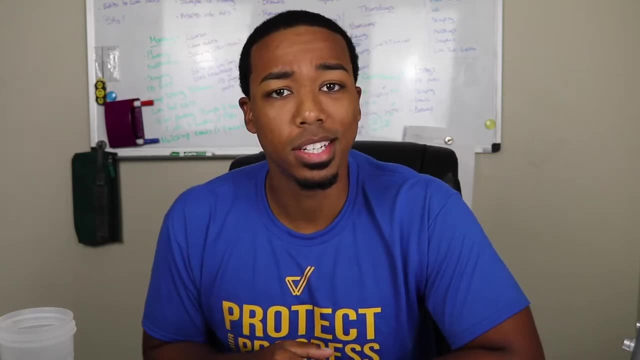 know what you're looking for. right, And now let's think about another example. Let's go ahead and think about, well, the whole analogy of you don't get in your car and drive unless you know where you're going- I mean, that's a pretty self-explanatory statement right Now, let's go ahead and apply. 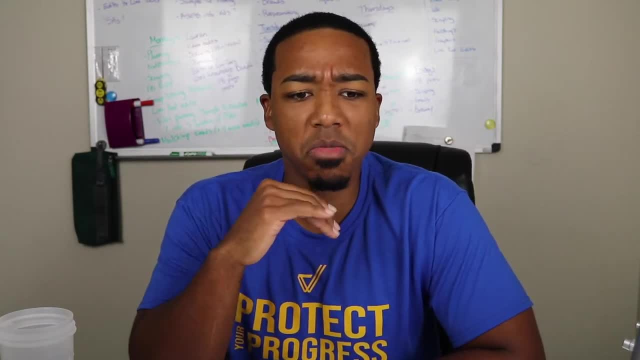 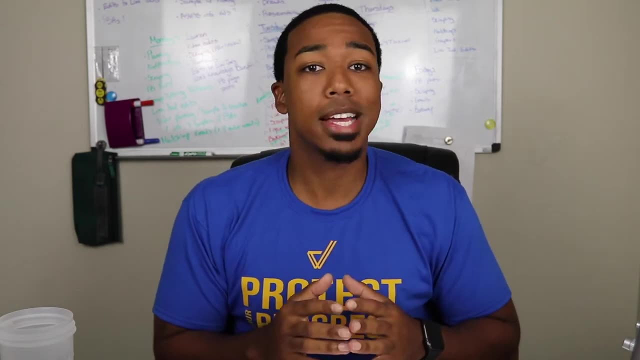 that to word problems. So let's go ahead and say: you know the average person- and this is a true statement, because I've been doing this for about 11 years now and I've seen this way too common Most people. what they do when they read a word problem is they get fixated on the numbers first. 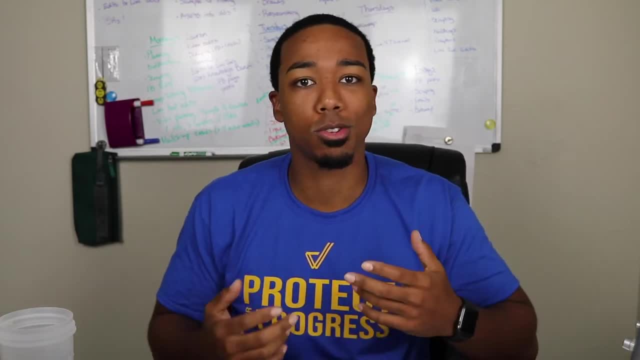 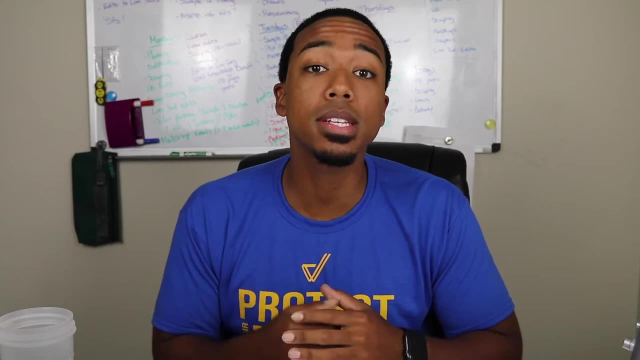 You know, they go straight to the numbers and they start calculating together with those numbers and then just hope for the best. Maybe single Hail Mary here and there, right, But the thing is that's not going to get you anywhere at all. And the reason, again, is because 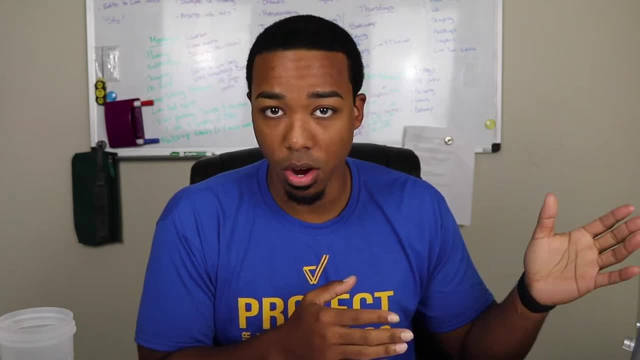 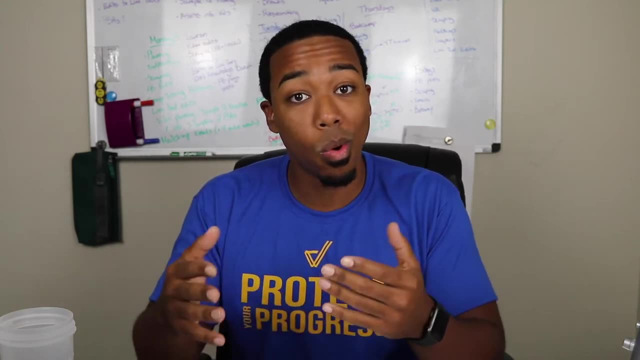 before you get in your car. typically, you know where you're going to go, You know what the destination is, You know where you're going, And so when you start a word problem, you need to understand what the question is, what you're answering, what you're trying to figure out. All. 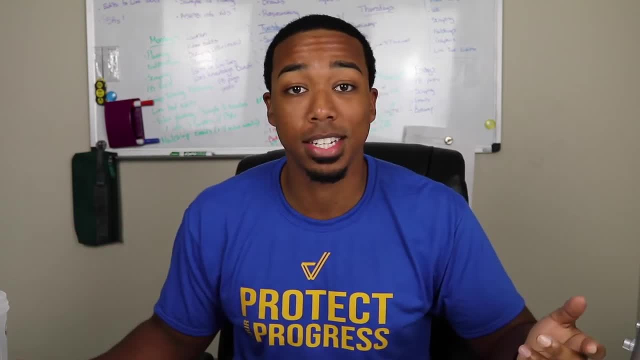 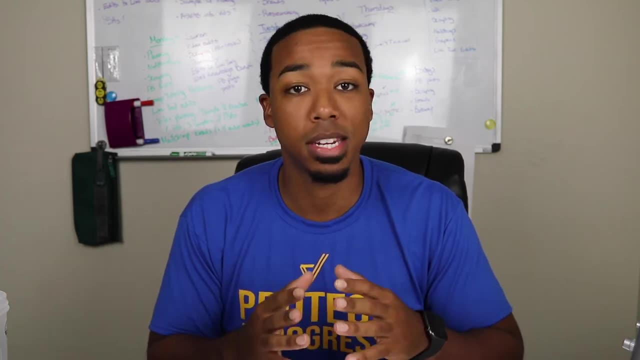 of the extra information. it's just extra information, It really is, until you know what its purpose is. So the numbers don't get fixated on those, Just get fixated on what the numbers mean at first. But before you even do that, again, you need to know where you're going. So let's go. 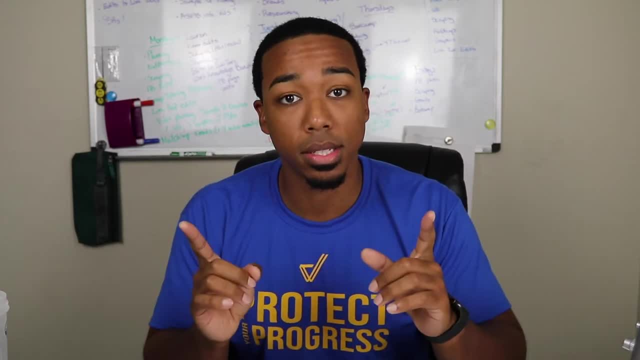 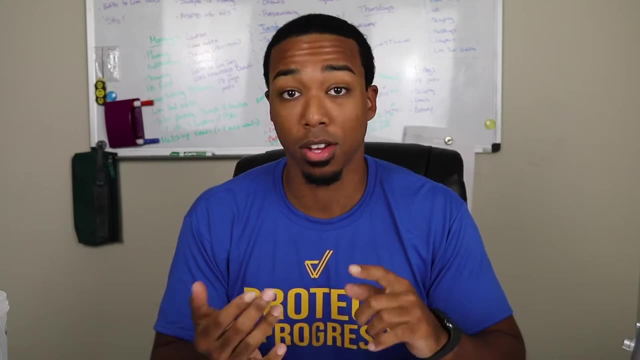 through the methodology You get in your car, but before you do that, you know where you're going. Great. Now, when you get in your car, you can't just speed off Because, remember, if you have a car, you know good and well that the car needs to warm up first, The oil needs to get hot And two. 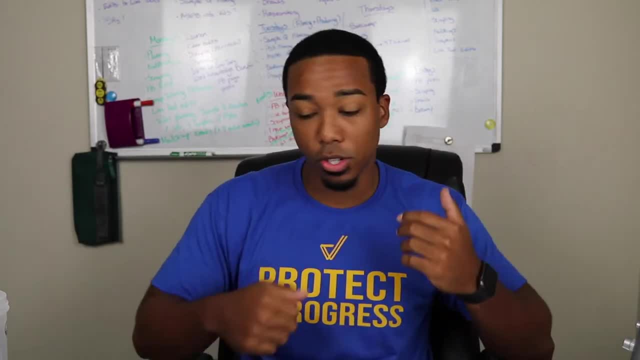 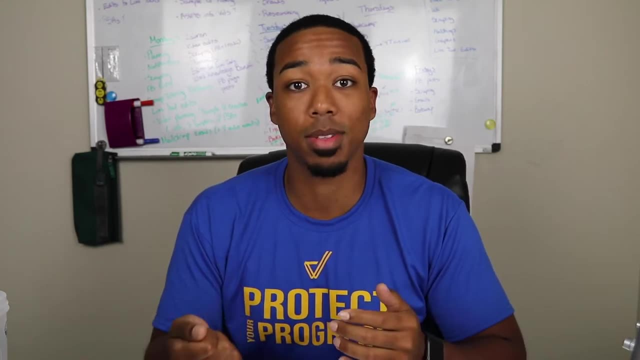 you need to go ahead and make sure that everything's all strapped up. You know your seat belt's on. You got to make sure that you warm the car up. You got to make sure that all these things are happening so that your car doesn't break down, Because I promise you, if you just slam the gas. 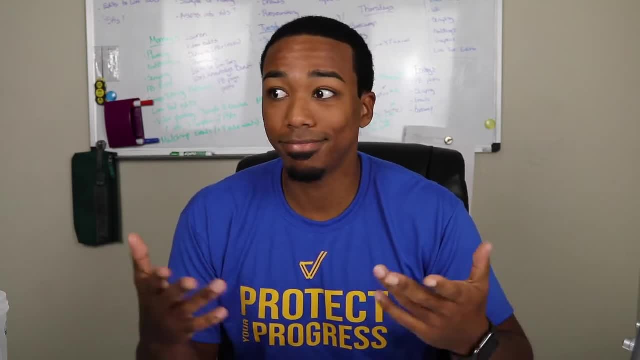 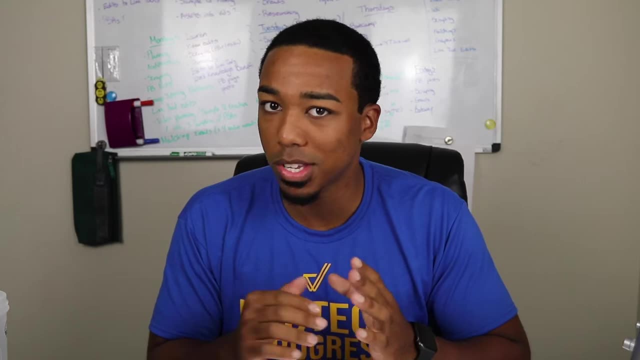 when you get in the car. well, guess what, If you keep doing that, after a while you know you're not going to get anywhere. You're not going to get to your destination, especially if you didn't really target where you're going to begin with. So I know this is a little lengthy of an analogy. 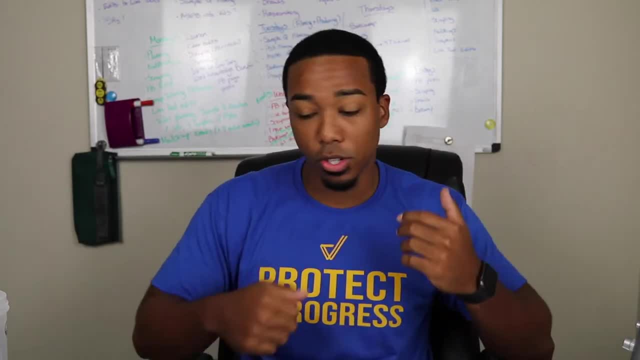 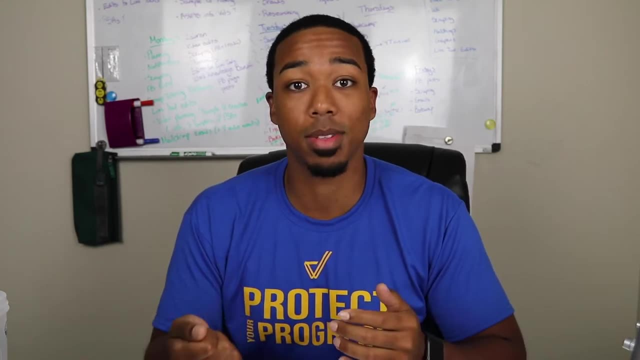 you need to go ahead and make sure that everything's all strapped up. You know your seat belt's on. You got to make sure that you warm the car up. You got to make sure that all these things are happening so that your car doesn't break down, Because I promise you, if you just slam the gas. 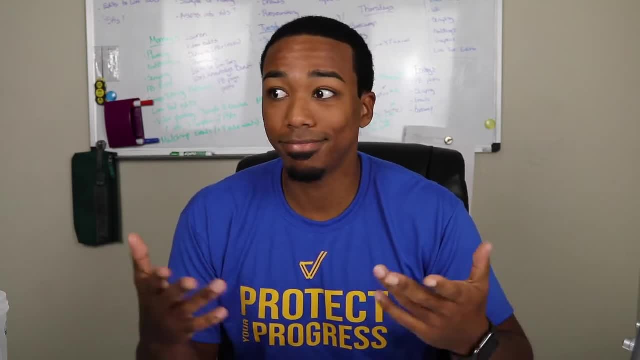 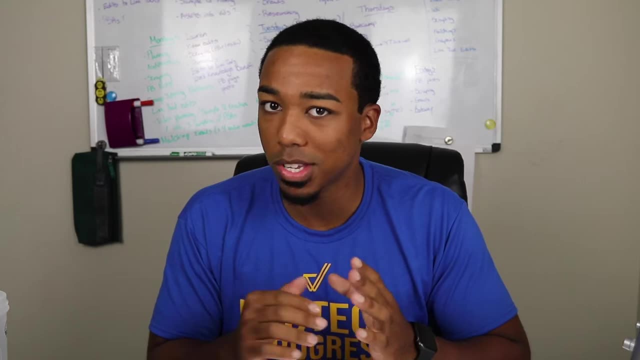 when you get in the car. well, guess what, If you keep doing that, after a while you know you're not going to get anywhere. You're not going to get to your destination, especially if you didn't really target where you're going to begin with. So I know this is a little lengthy of an analogy. 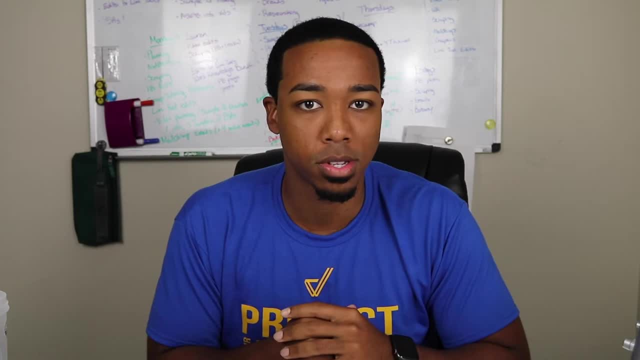 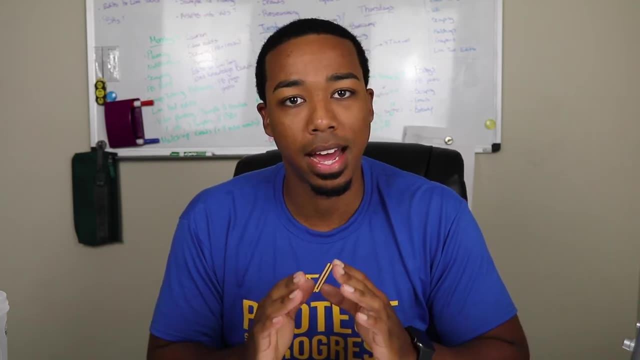 but guess what? This is going to help you out tons. So back to the word stuff. So with the word problem again. first things, first read the question, Highlight those keywords. You have to analyze, You have to let yourself warm up, You have to understand what it is that you're. 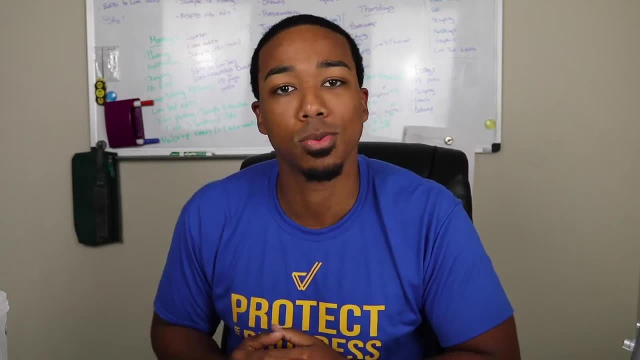 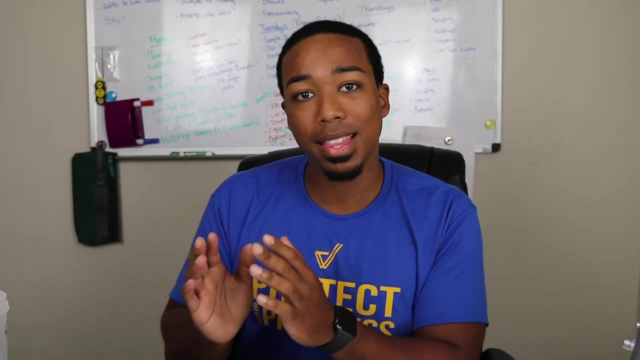 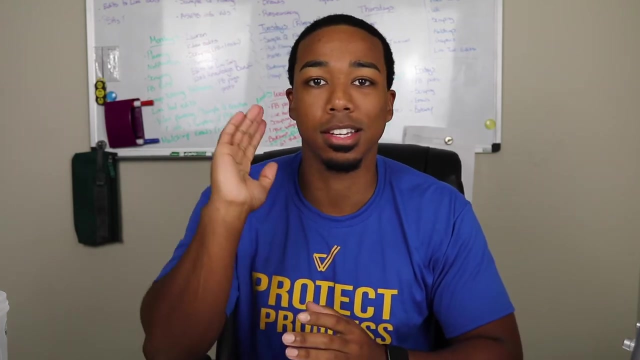 connecting in terms of the information, And again I'm going to show you an example of how this works in a moment. But again you have to understand what the question is, Highlight those keywords and then make that connection before you go in and dive into the information, before you start hitting the gas and slamming that thing and going. 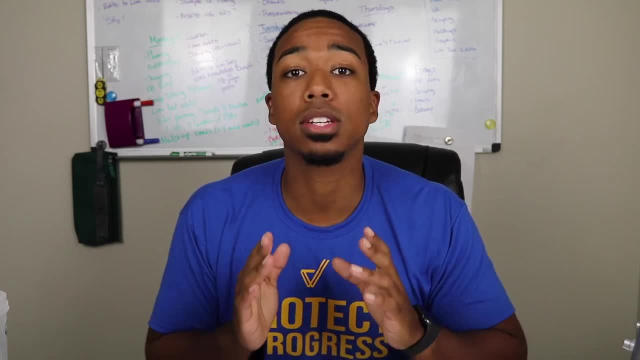 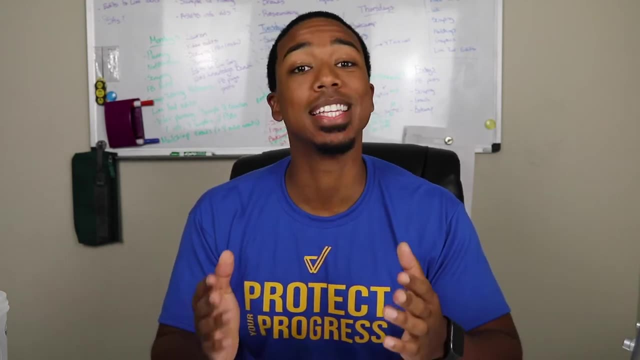 100 miles an hour, Because, again, the numbers don't matter unless you know what they mean. One more time: The numbers don't matter unless you know what they mean. I kind of say that a million times. So let's get back to it Once. you highlight those keywords and you make that. 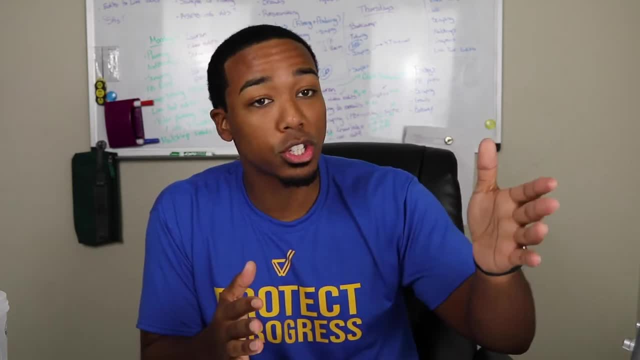 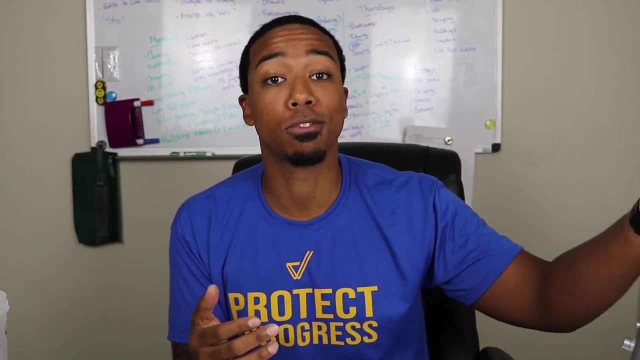 connection, then you have a better sense of the direction. You have to remember this are your�IOS. You have to remember that you have a purpose, a mission, that you're going in because you know what the goal is and you know what information. 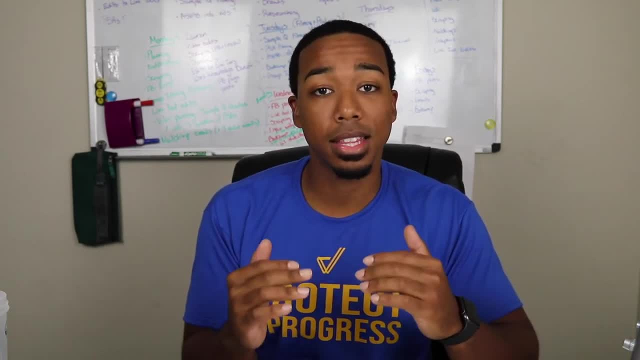 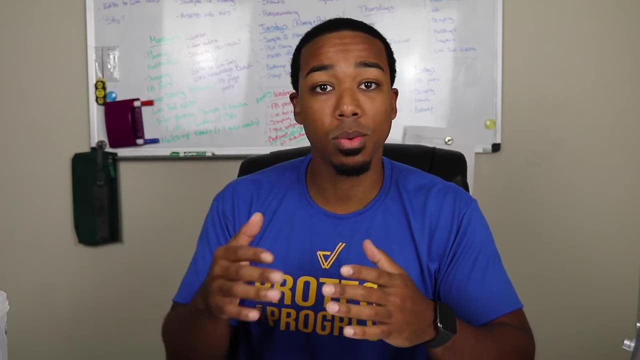 you have, which allows you to paint that picture for yourself. So again, in terms of driving, you've got to get in your car, you've got to let that car warm up and you have to identify where you're going and how you're going to get there. That's the same thing in math. 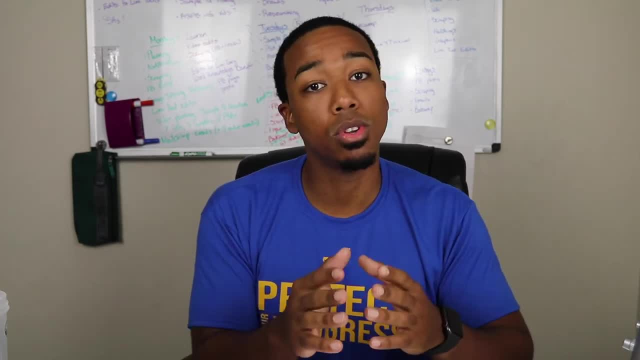 Again, keywords that use the information to make the connection and make your plan. So then, in your car, once you know where you're going, how to get there and why you're doing it точно, can use your Geralasilante Setups to unlock it for you as well. 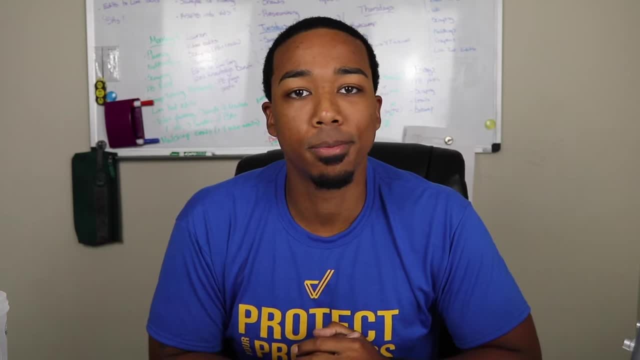 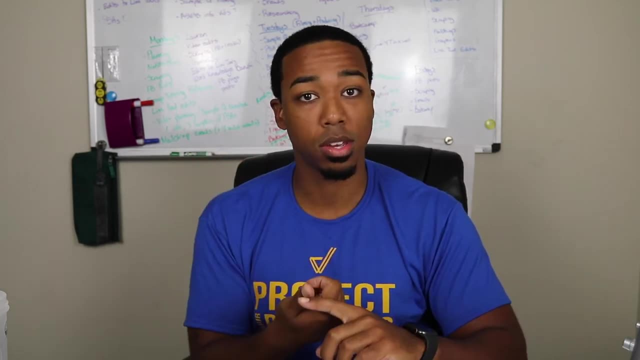 you just drive off because your car is warm, it's all good, And there you go. Same thing with word problems in math. You want to analyze first, give yourself that time to really get those gears going in terms of those keywords, And then you look at the numbers and you say, okay, that number. 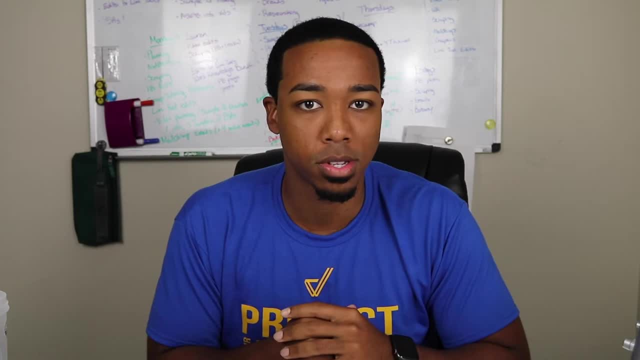 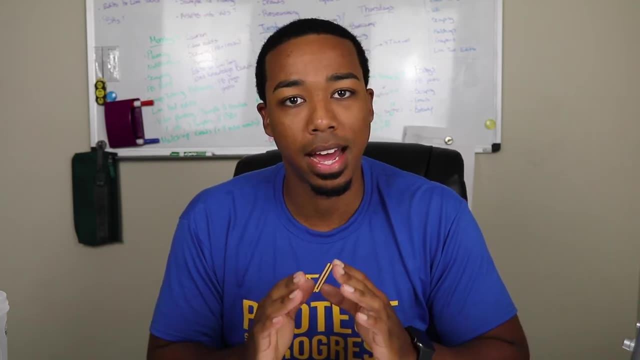 but guess what? This is going to help you out tons. So back to the word stuff. So with the word problem again. first things, first read the question, Highlight those keywords. You have to analyze, You have to let yourself warm up, You have to understand what it is that you're. 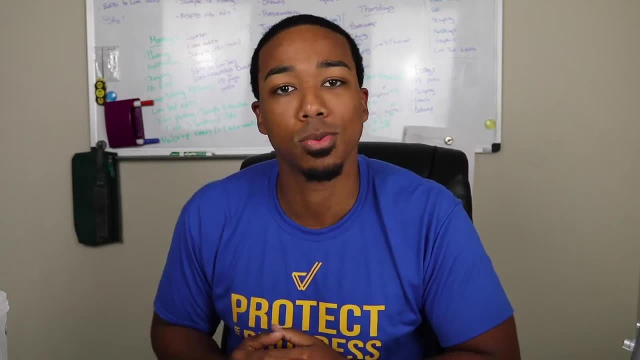 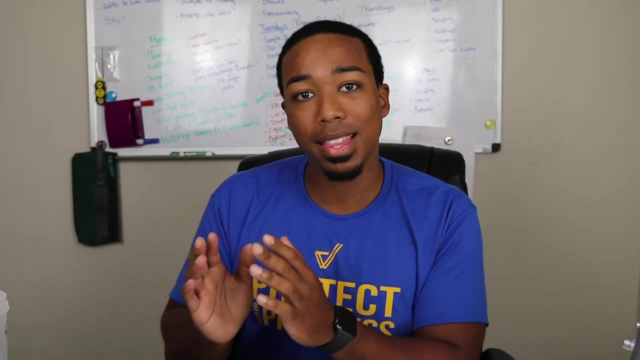 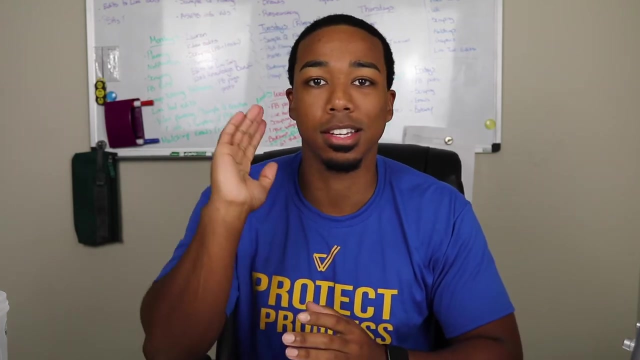 connecting in terms of the information, And again I'm going to show you an example of how this works in a moment. But again you have to understand what the question is, Highlight those keywords and then make that connection before you go in and dive into the information, before you start hitting the gas and slamming that thing and going. 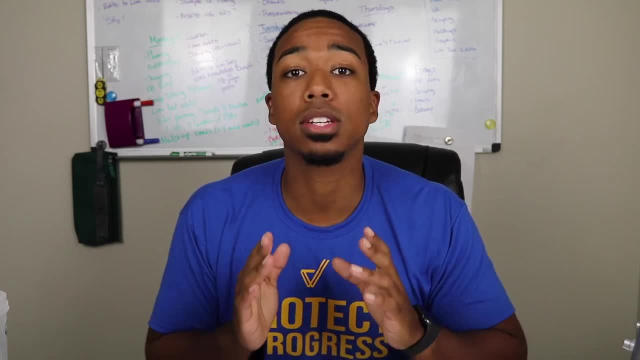 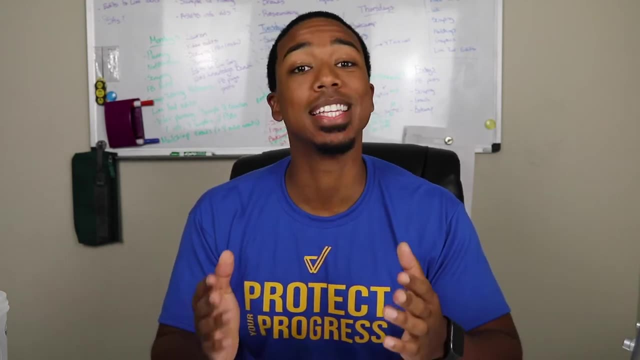 100 miles an hour, Because, again, the numbers don't matter unless you know what they mean. One more time: The numbers don't matter unless you know what they mean. I kind of say that a million times. So let's get back to it Once. you highlight those keywords and you make that. 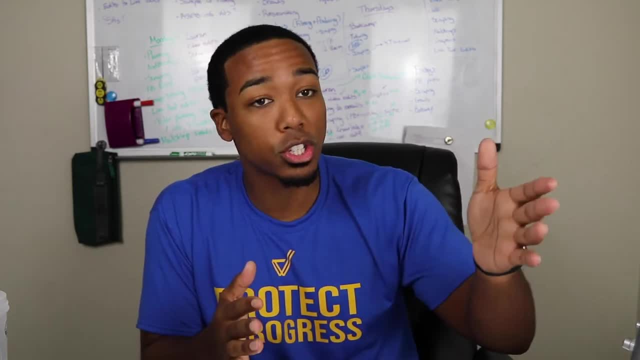 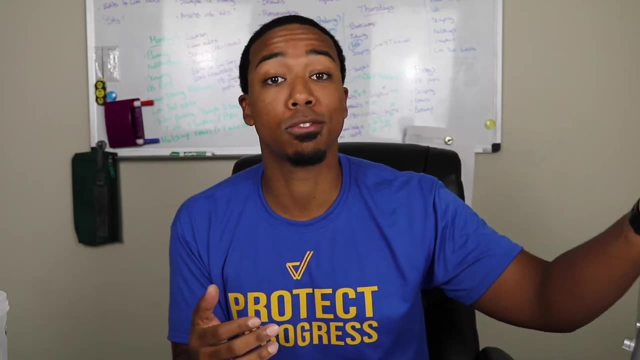 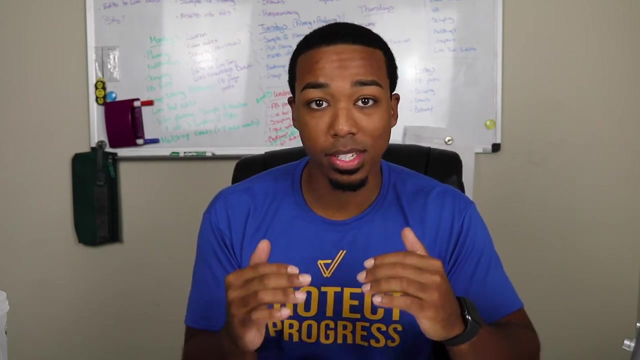 connection, then you have a better sense of the direction, Because you know what the goal is and you know what information you have which allows you to paint that picture for yourself. So, again, in terms of driving, you got to get in your car, you got to let that car warm up and you have to identify. 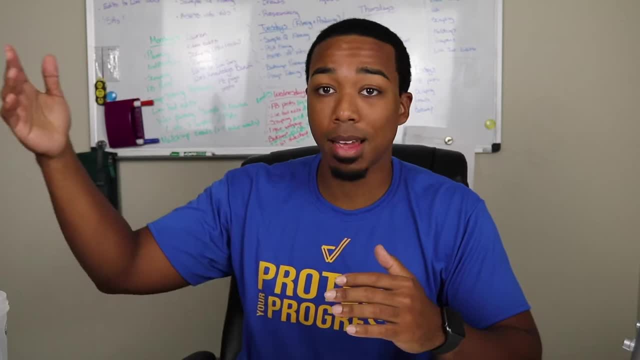 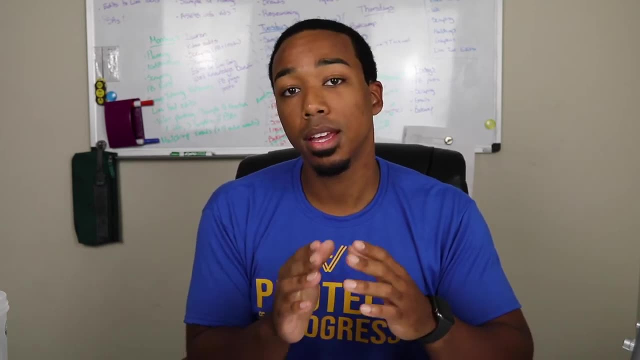 where you're going and how you're going to get there. That's the same thing in math. Again, key words: Use the information to make the connection and make your plan. So then in your car, once you know where you're going, how to get there and why you're doing it. 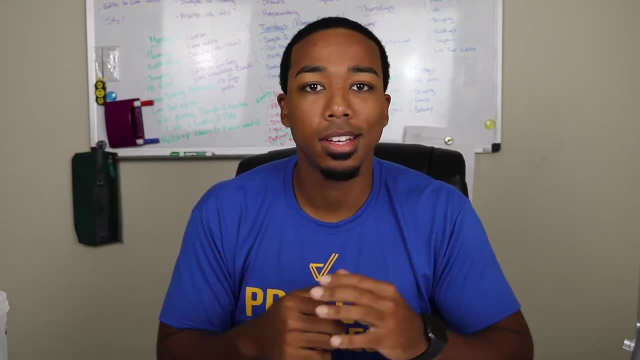 boom. Then you know where to go and why you're doing it. You're going to find it. You're going to find it. You know what you're going to get there And you know what you're doing. You got to, you just drive off because your car is warm, it's all good And there you go. Same thing with word. 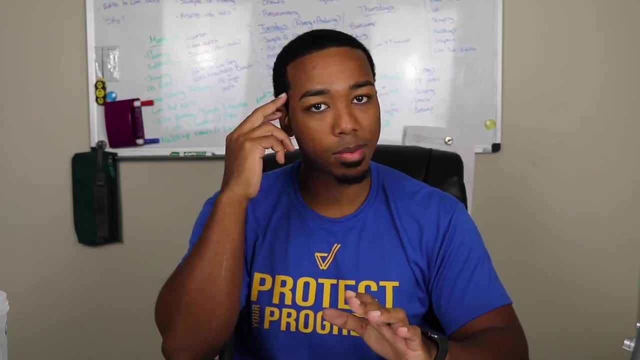 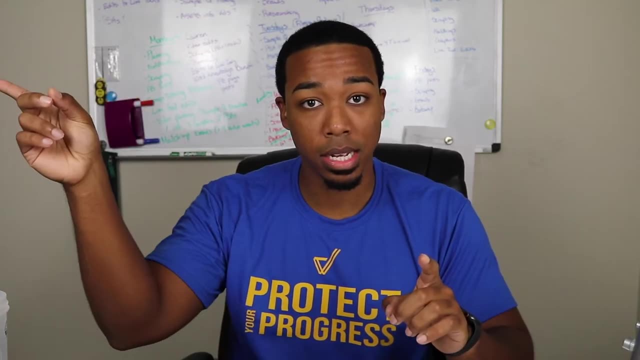 problems in math. You want to analyze, first, give yourself that time to really get those gears going in terms of those keywords, And then you look at the numbers and you say, okay, that number represents what I needed And this number over here represents another piece of information that 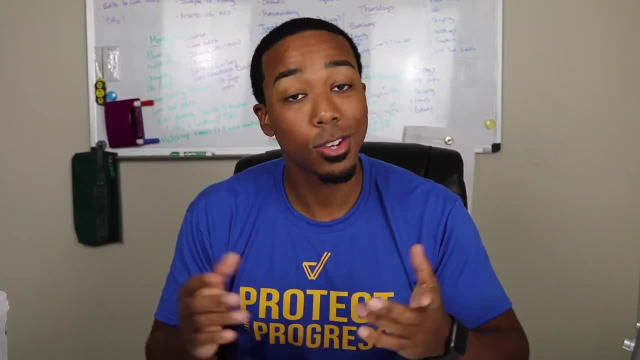 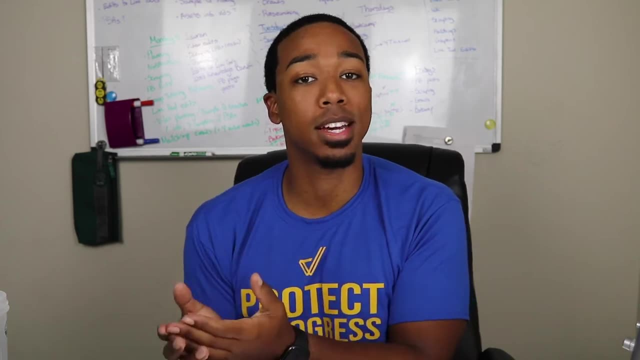 I can use. Oh, look at that, That over there is extra information. Don't you hate it when you are falling for that trap of using information that you don't need? Everybody does. And the thing is, it happens because, again, we're not disciplined in terms of analyzing before we approach the 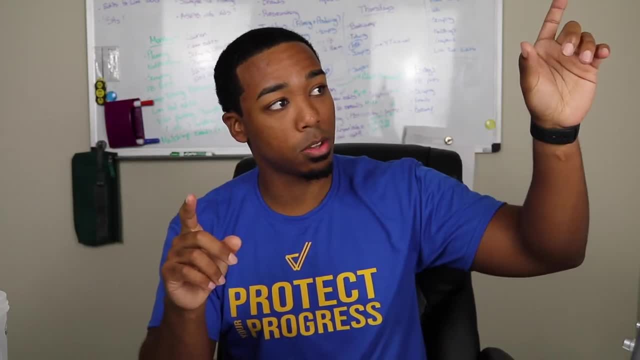 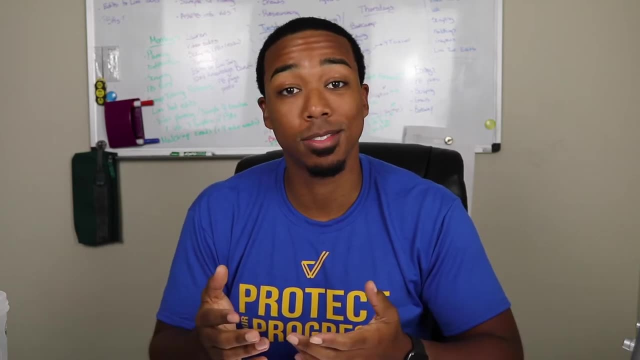 represents what I needed, And this number over here represents another piece of information that I can use. Oh, look at that. That over there is extra information. Don't you hate it when you are falling for that trap of using information that you don't need? Everybody does, And the thing is: 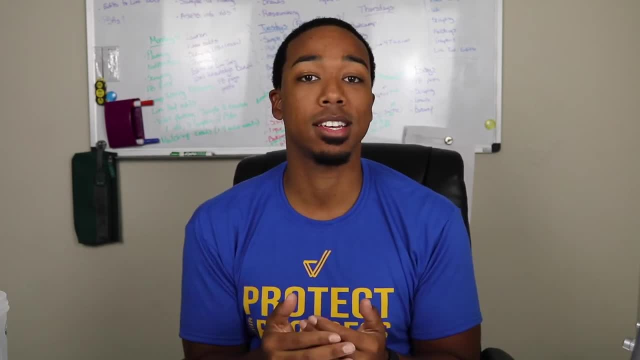 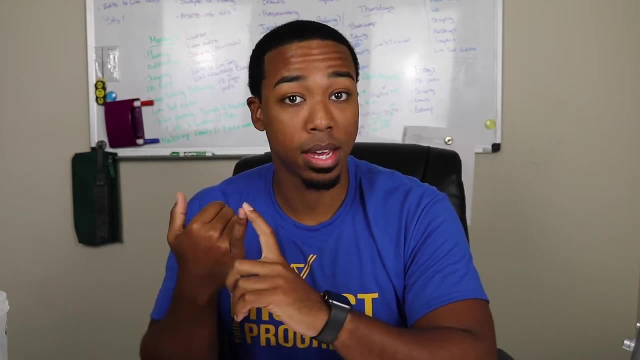 it happens because, again, we're not disciplined in terms of analyzing before we approach the problem. So when you analyze, that gives you the opportunity to again search through your memory and say, okay, what does this all mean? What do these keywords mean? What information might I need? 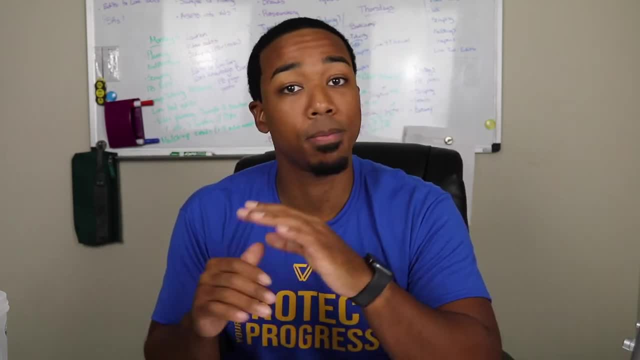 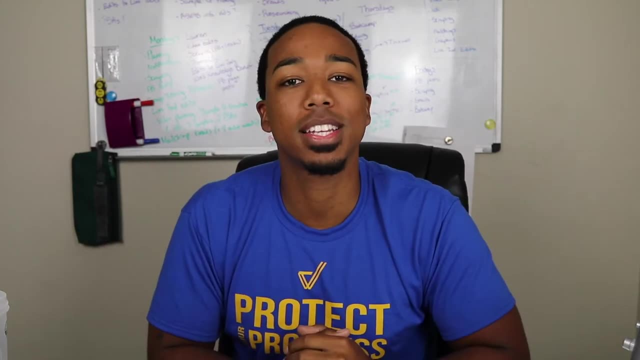 to answer this question. Now I'm going to go in, look at those keywords, every instance of that, and figure out everything that matches up And once you have that boom, then you can go ahead and attack the problem like the animal you are and then get that problem right and move on forward. 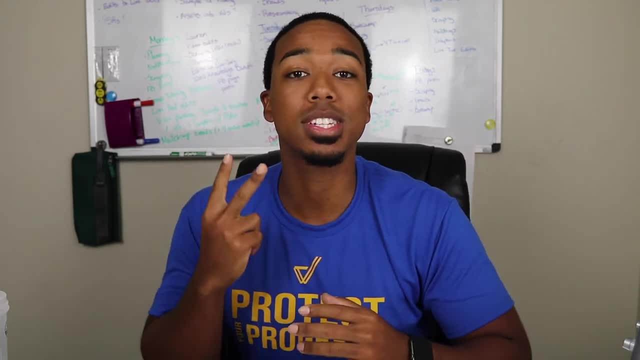 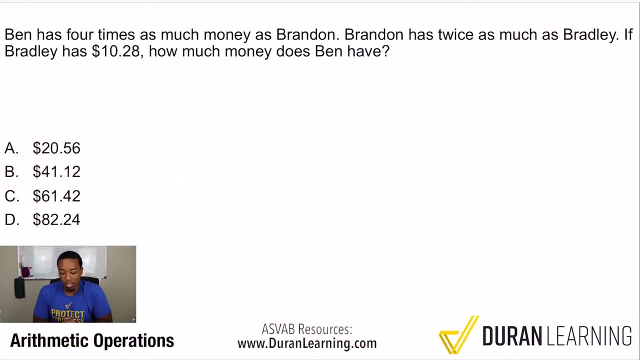 So, with that said, enough of me talking, we're going to go ahead and look at two example problems. So let's go ahead and dive right in Number one here. Ben has four times as much money as Brandon. Brandon has what? 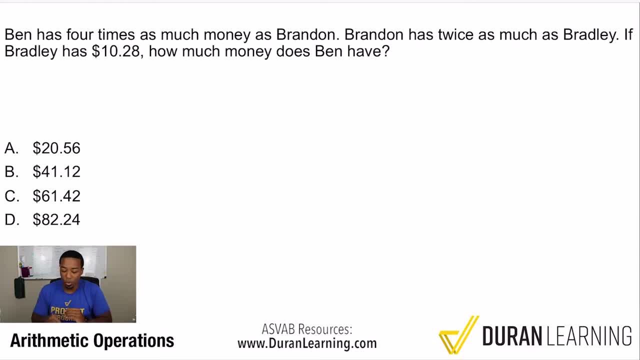 did I say: Read the question first, right? So we're going to ignore everything there, Ignore all of this stuff over here, Just ignore it, Just go straight to the question statement. And that question statement is: how much money does Ben have? That is our key here: How much money does. 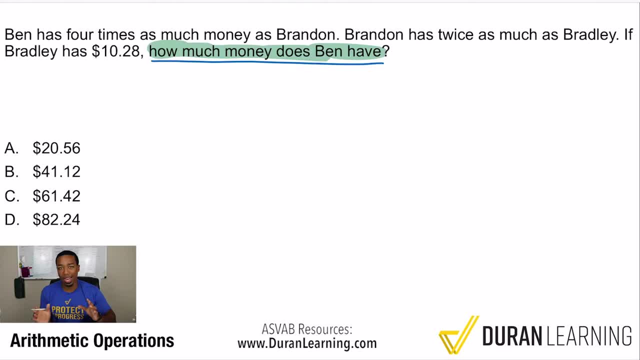 Ben have. That is what we're going to talk about. So let's go ahead and look at two examples. Remember that four is exactly what we're looking for. That's exactly what we're looking for. So let's just highlight some things here. We're looking for how much money that Ben has. Those 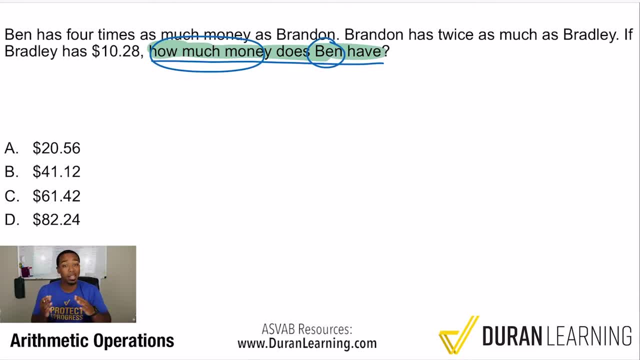 are the keywords money and Ben, How much money Ben has, That's it. So, whoever this Ben character is, we're looking for how much money he has. So we're looking for how much money Ben has. Again, that's your only concern. That's your only concern. So then, look, now that you understand, 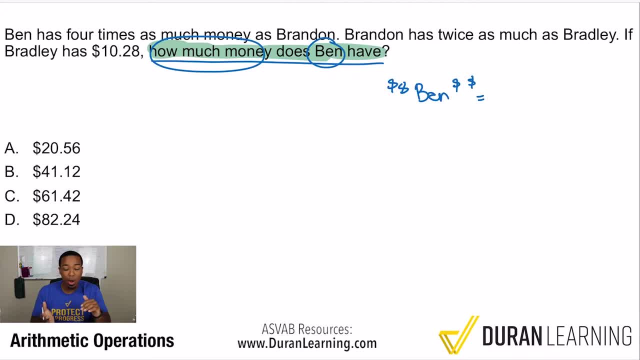 that money ben has. that's the key to the question. now we can go back into the question and look at every instance that talks about ben and his money. that way, we can make connections to the problem and only use the information that we need again. that's what it's all about: wasting less time. 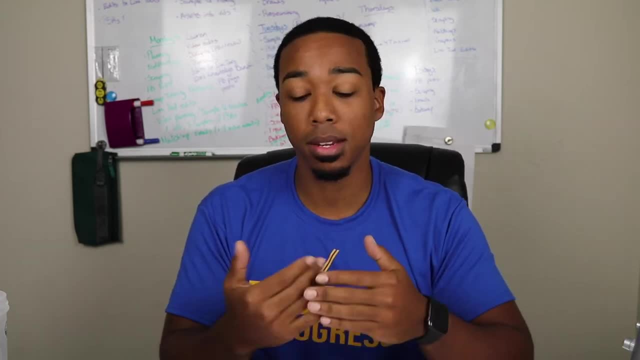 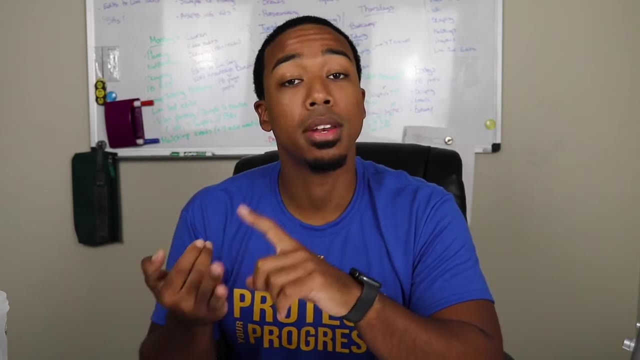 problem. So when you analyze, that gives you the opportunity to again search through your memory and say, okay, what does this all mean? What do these keywords mean? What information might I need to answer this question? Now I'm going to go in look at those keywords every instance of that. 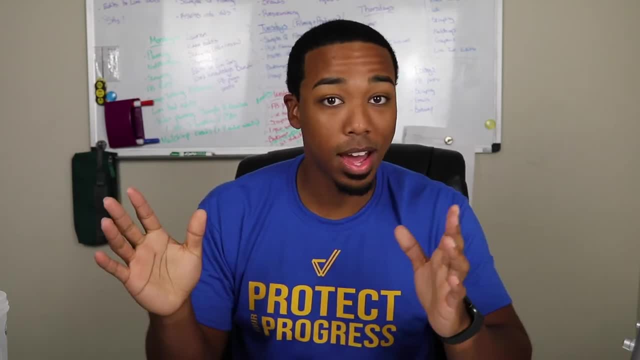 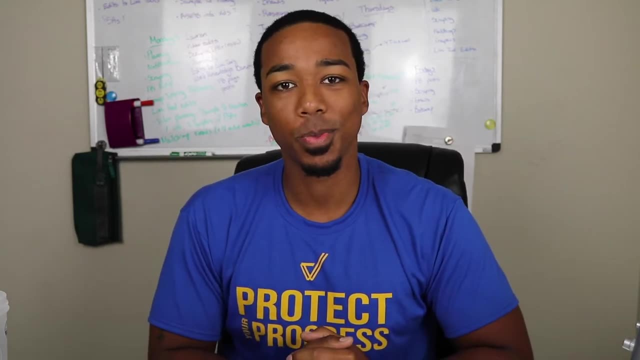 and figure out everything that matches up, And once you have that boom, then you can go ahead and attack the problem like the animal you are, and then get that problem right and move on forward. So, with that said, enough of me talking. we're going to go ahead and look at two example problems. So let's go ahead. 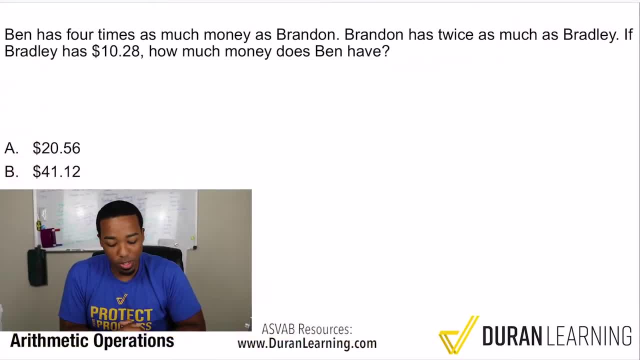 and dive right in Number one here. Ben has four times as much money as Brandon Brandon has. what did I say? Read the question first, right? So we're going to ignore everything there. Ignore all of this stuff over here, Just ignore it. Just go straight to the question statement And that. 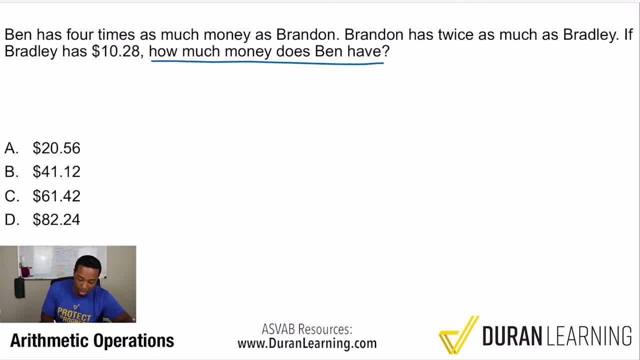 question statement is: how much money does Ben have? That is our key here. How much money does Ben have? That is what we're going to talk about. So let's go ahead and look at two examples. So number one: this is a key question that Ben has. So number two: this is a key question that Ben 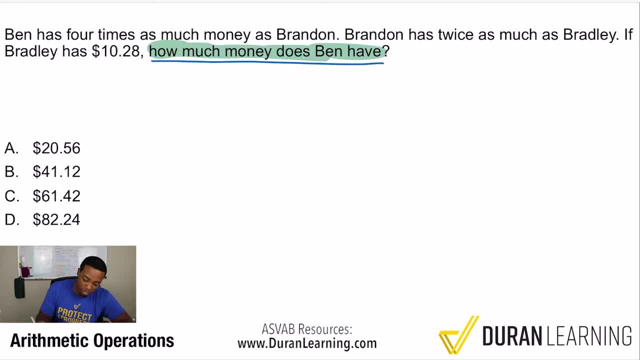 has. That is what we're looking for. All right, that's exactly what we're looking for. So let's just highlight some things here. We're looking for how much money that Ben has. Those are the key words: money and Ben. How much money Ben has, that's it. So, whoever this Ben character is, 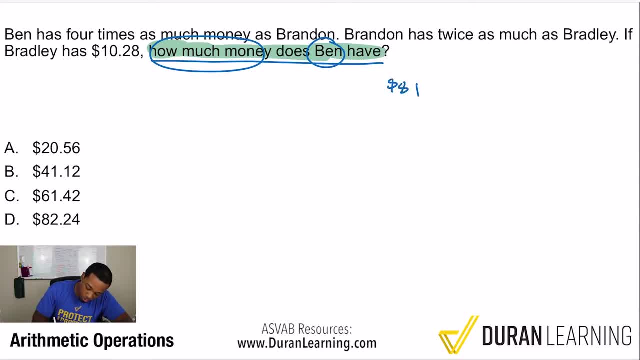 we're looking for how much money he has, All right. So we're looking for how much money Ben has, Again, that's your only concern. That's your only concern, All right. So then look now that you understand that, All right. 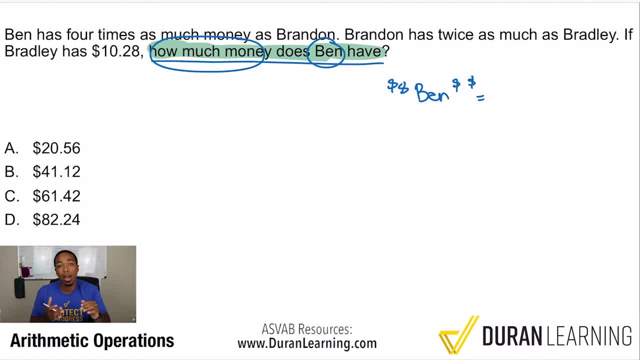 money Ben has. That's the key to the question. Now we can go back into the question and look at every instance that talks about Ben and his money. That way, we can make connections to the problem and only use the information that we need. Again, that's what it's all about: wasting less time. 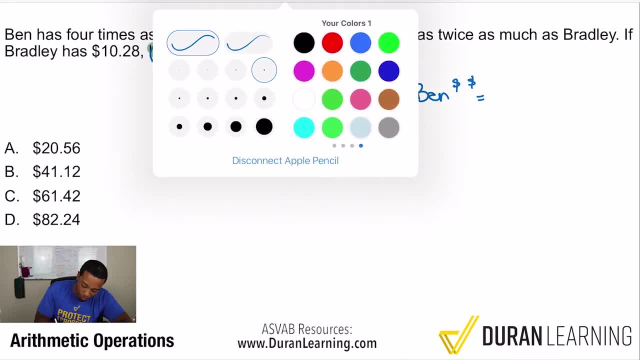 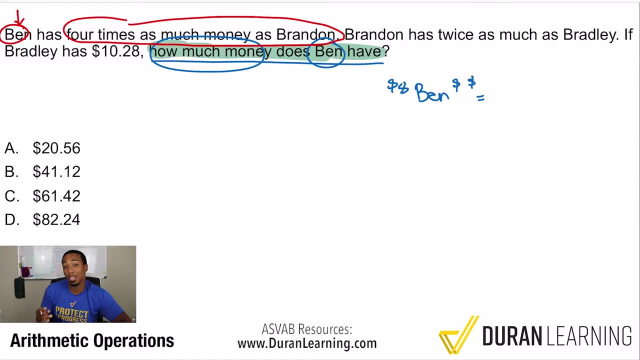 So here we go. If I'm going ahead and highlighting everything that I need here, well, we're looking for everything that includes Ben. There's Ben, right there. Great Ben has four times as much money as Brandon. Okay, So really, what does that mean? Well, that doesn't give me an exact 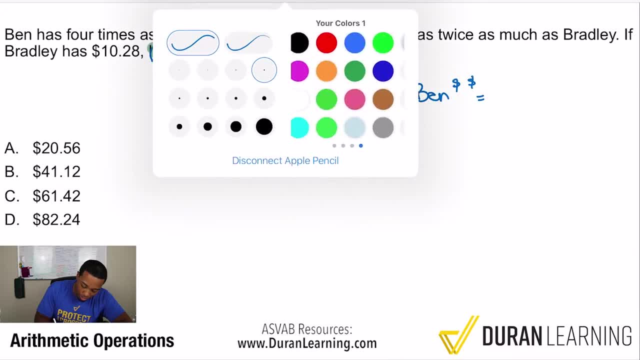 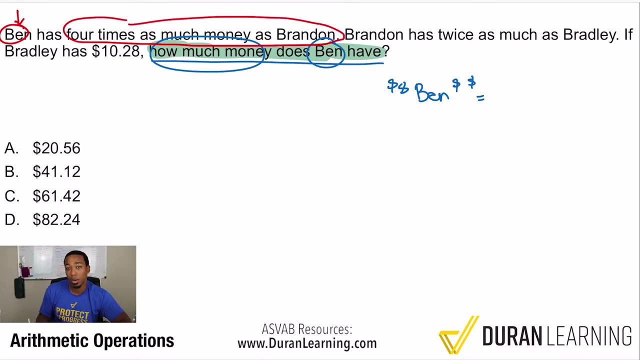 so here we go. if i'm going ahead and highlighting everything that i need here, well, we're looking for everything that includes ben. there's ben, right there. great ben has four times as much money as brandon. okay, so really, what does that mean? well, that doesn't give me an exact number for ben, right? 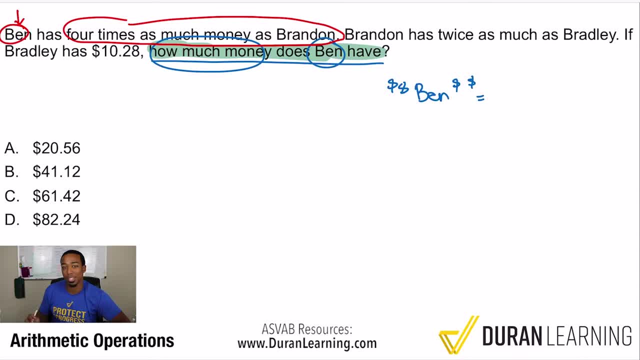 it doesn't, but this sounds like the type of problem where you're going to have to connect a bunch of pieces of information and that's okay. you just have to be patient with yourself and let the problem develop. so we have ben and he has four times as much money as brandon. so ben, what i know. 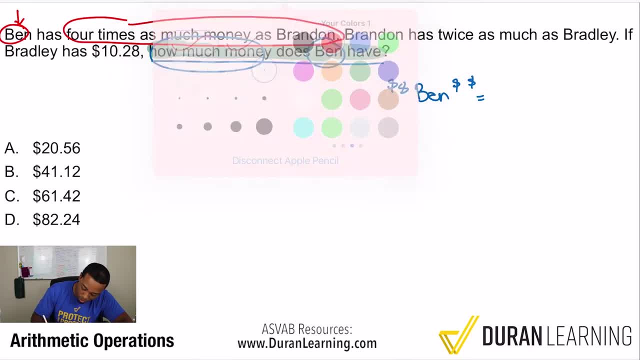 about ben right now again, is he has actually go back to red here. he has four times as much as brandon. all right, so that doesn't get me the answer, but it looks like i'm going to have to know a little bit more about brandon if i want ben, right, so let's go ahead and find some more information here. what 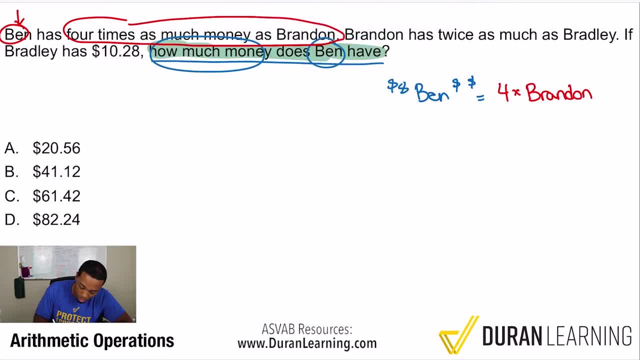 do we have? well, additionally, here we see that we have brandon right there and he has twice as much as bradley. so, brandon, brandon, he equals twice as much as bradley. all right, so now this is going down a rabbit hole, right, but we're still focused, we still know. 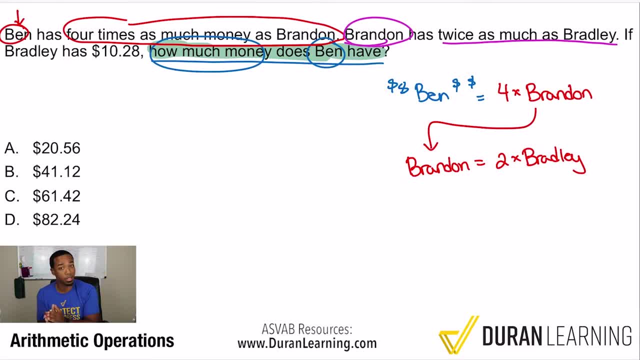 that ben is connected to brandon and brandon is connected to bradley. now let's see what bradley. if there's any other information on him, oh for sure, bradley has 10.28. so let me just go ahead and change bradley's color here to purple, and i see here that again, bradley has. 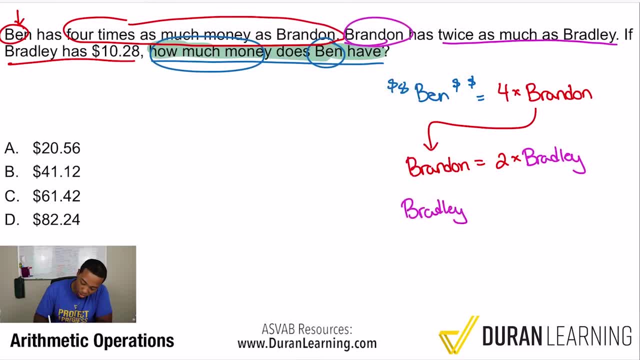 and again, you're not always writing this out, you're not always writing this out, but i'm just writing it out to help you visualize. all right, i want to help you visualize because again we started with the question: we want to know how much money we have and we're going to have to. 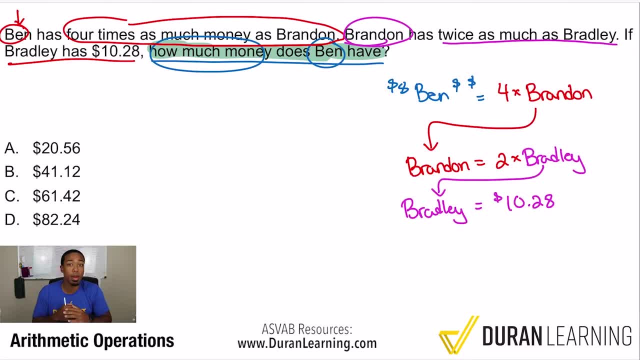 figure out how much money ben has- all right money ben has. so we're going straight back into the problem and we said: all right, ben is four times as much as brandon. and then we also found out that brandon is twice as much as bradley. so we want to go ahead and take bradley, which we now 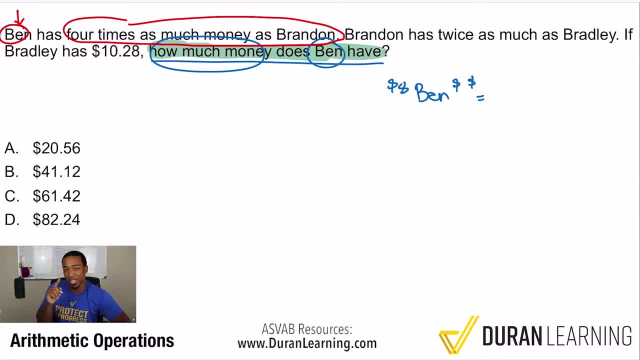 number for Ben? right, It doesn't, But this sounds like the type of problem where you're going to have to connect a bunch of pieces of information And that's okay. You just have to be patient with yourself and let the problem develop. So we have Ben and he has four times. 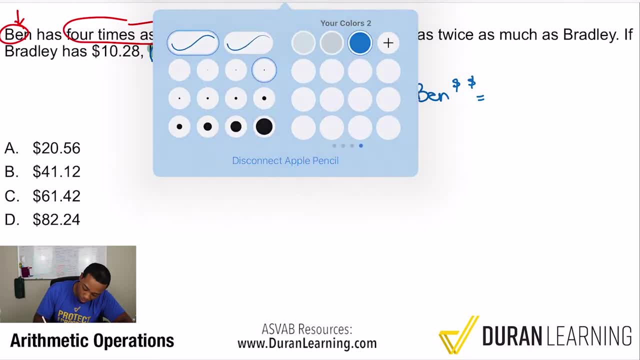 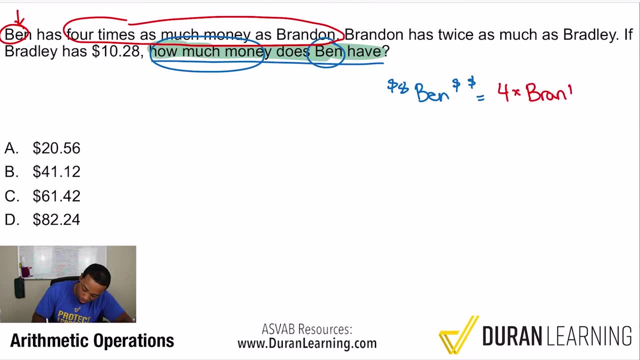 as much money as Brandon. So, Ben, what I know about Ben right now again is he has actually- let me go back to red here- He has four times as much as Brandon. All right, So that doesn't get me the answer, but it looks like I'm going to have to know a little bit more. 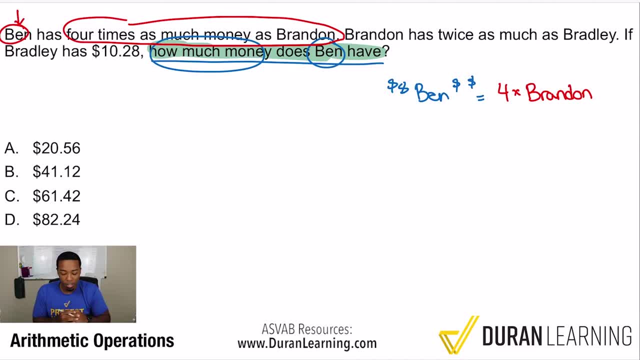 about Brandon if I want Ben, right. So let's go ahead and find some more information here. What do we have? Well, additionally, here we see that we have Brandon right there and he has twice as much as Bradley. So Brandon. 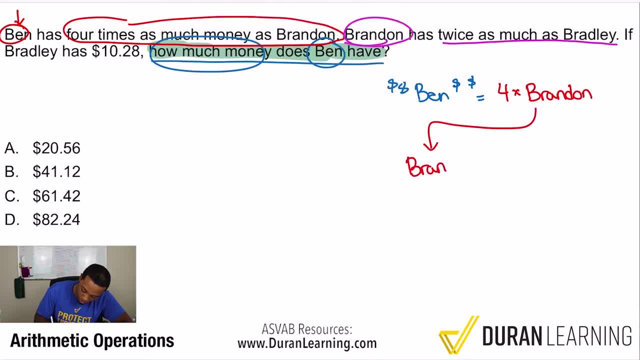 Brandon. he equals twice as much as Bradley. All right, So now this is going down a rabbit hole, right? But we're still focused. We still know that Ben is connected to Brandon and Brandon is connected to Bradley. Now let's see what Bradley 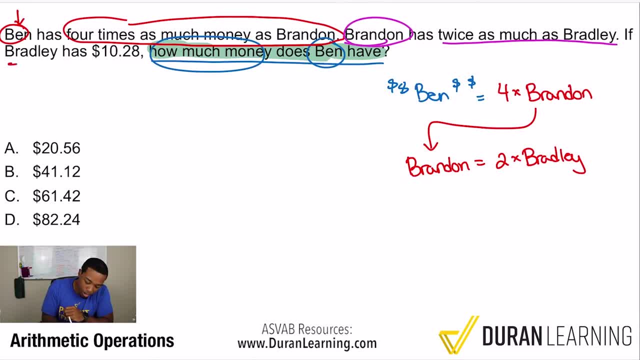 if there's any other information on him. Oh for sure, Bradley has $10 and 28 cents. So let me just go ahead and change Bradley's color here to purple, And I see here that again Bradley has. and again, you're not always writing this out. You're not always writing this out. 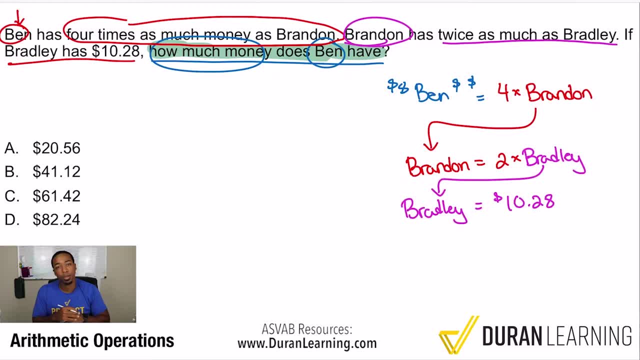 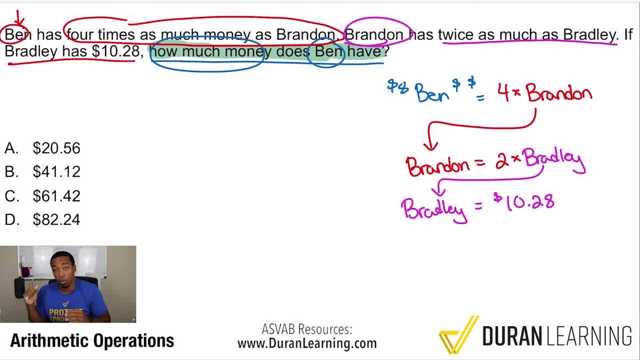 We want to know how much money Ben has- All right Money Ben has. So we're going straight back into the problem And we said, all right, Ben is four times as much as Brandon. And then we also found out that Brandon is twice as much as Bradley. So we want to go ahead and take Bradley. 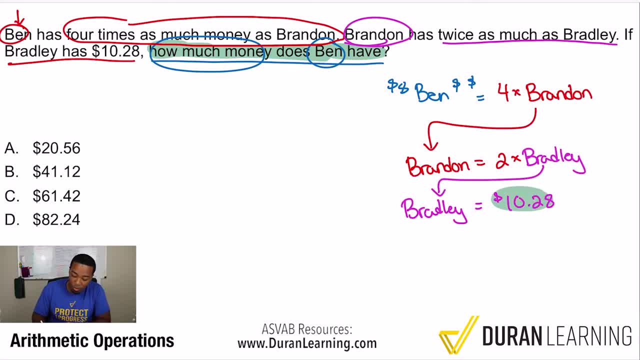 which we now have as $10 and 28 cents. If we multiply that by two, we get Brandon. And then, whatever Brandon is, we multiply by four and we get Ben. So this all needs to happen within 20, 30 seconds. a quick like quick, quick, quick. The majority of your time in a problem is setting. 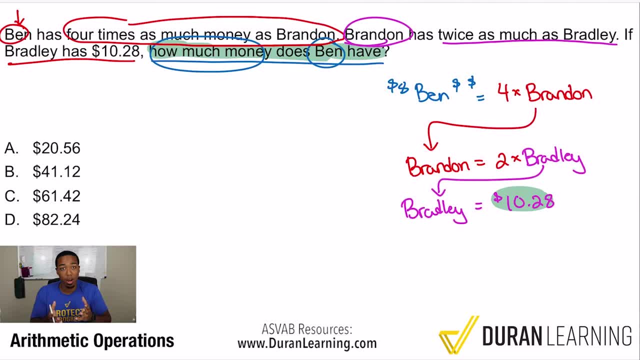 it all up. So this needs to happen as quickly as possible, Nowhere you know, anywhere between 20 and 40 seconds because the actual calculation I'm going to tell you right now. if you're not quick at calculating, you need to be download a mental math app or do whatever you need to do to practice. 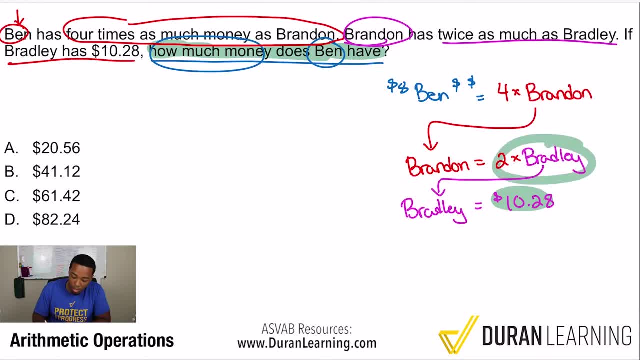 have as ten dollars and 28 cents. if we multiply that by two, we get brandon. and then, whatever brandon is, we multiply by four and we get ben. so this all needs to happen within 20, 30 seconds. like quick, like quick, quick quick- the majority of your time, and a problem is setting it all up. 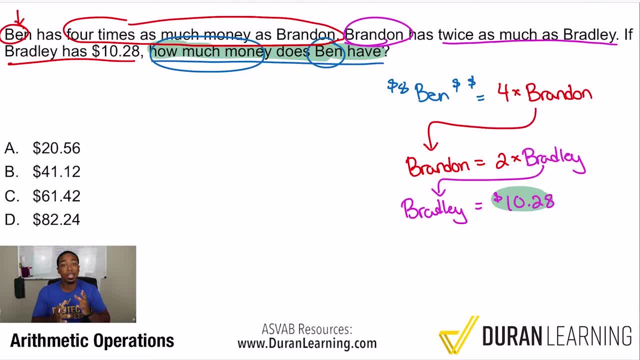 this needs to happen as quickly as possible. nowhere, you know, anywhere between 20 and 40 seconds because the actual calculation i'm going to tell you right now. if you're not quick at calculating, you need to be download a mental math app or do whatever you need to do to practice. 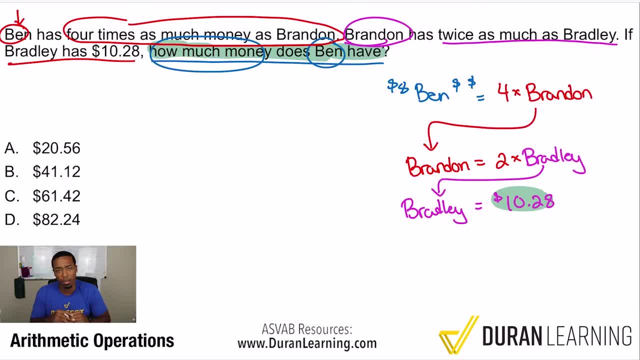 consistently, so that the actual calculation is not what holds you back, because you can multiply, add, subtract and divide. we know how to do that. let's do it quicker now. so here's another way that we can shorten the time that this problem is going to take us, because, again, we could definitely 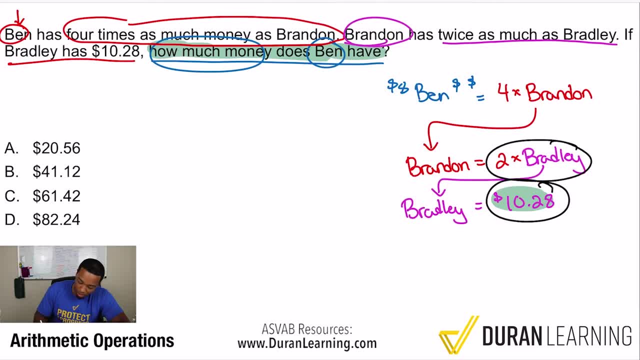 start with ten dollars and twenty eight cents, multiply it by ten dollars and twenty eight cents by two, then multiply by four. we can definitely do that. but ask yourself this question: if you multiply something by two and then you multiply that thing by four, what are you really doing? well, you're. 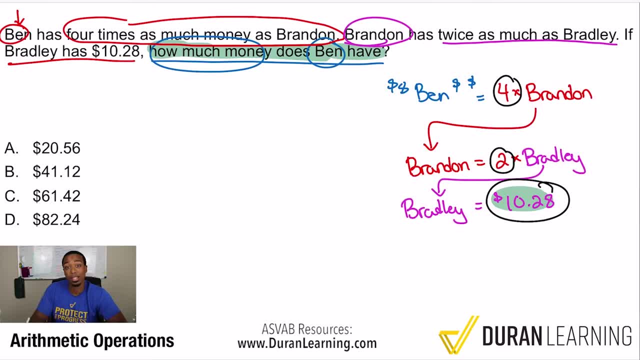 multiplying by eight, because times two times four, that's the same thing as times eight. so you could end up going again the 10, 28 you can get. multiply it by two, then by four, or you can just straight up multiply it by eight and save a lot of time. so i'm here to show you exactly how you can save that. 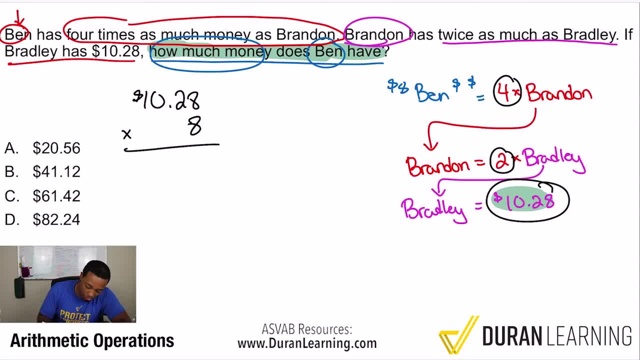 time, and here it is, by eight, ten, twenty, eight times eight. you can go ahead and just do that. eight times eight is 64, six two times eight is 16 plus six is 22, then zero times eight, that ends up being zero. put the two there and then you have the one times eight, which is eight, and so you have eighty two dollars, and 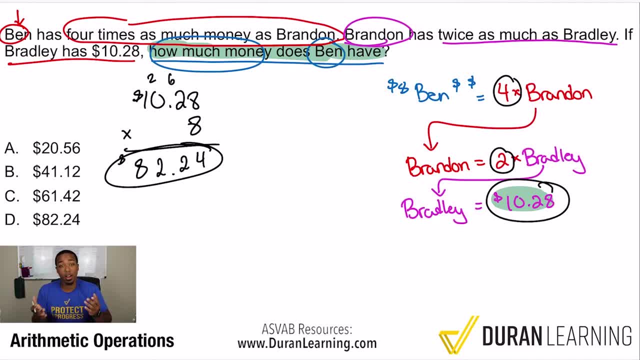 twenty four cents. that's what we end up with and that represents our final answer, because we ended up setting ourselves up. we started with the given information to connect it to what we needed to figure out and we ended up with the given information and we ended up with the given. 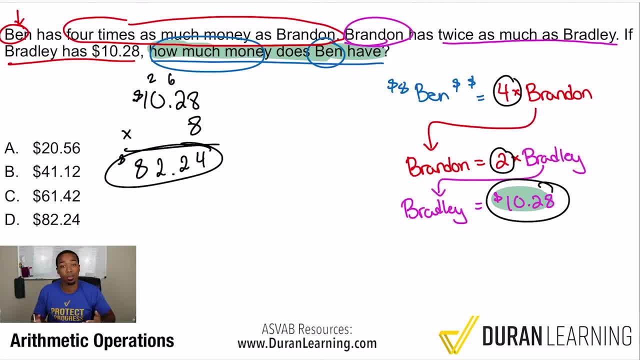 information and once we had that set up, boom, then calculate, then go to town. the last thing you need to do is calculate, guys. the last thing, the first thing you need to do is just worry about the question itself, because there's no point in looking at the numbers if you don't know what. 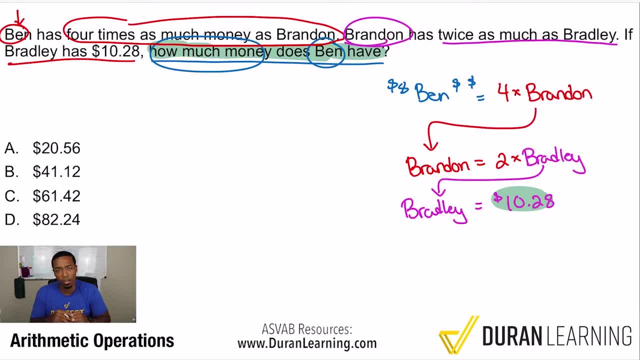 consistently, so that the actual calculation is not what holds you back, because you can multiply, add, subtract and divide. We know how to do that. Let's do it quicker now. So here's another way that we can shorten the time that this problem is going to take us, Because, again, we could. 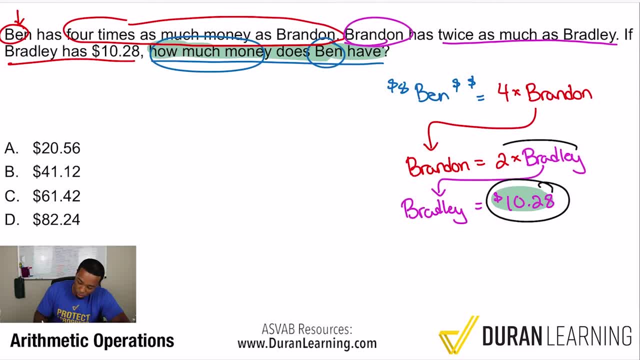 definitely start with $10 and 28 cents. So we're going to multiply it by two, then multiply it by four. We can definitely do that, But ask yourself this question: If you multiply something by two and then you multiply that thing by four, what are you really doing? Well, you're multiplying by eight because times two times four. 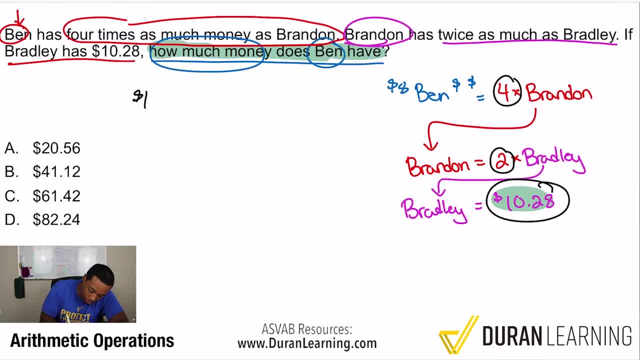 that's the same thing as times eight, So you could end up going again the 10, 28,. you can get. multiply it by two, then by four, or you can just straight up multiply it by eight and save a lot of. 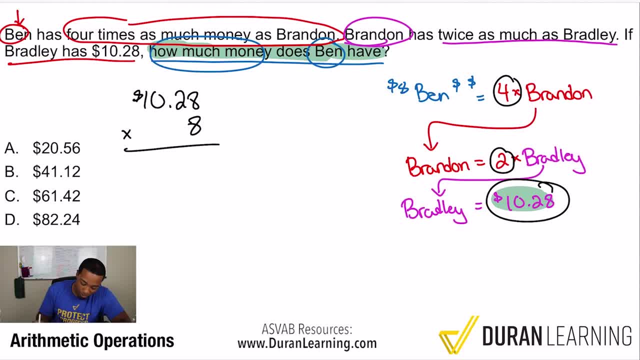 time. So I'm here to show you exactly how you can save that time. And here it is: By multiplying by eight, 10, 28 times eight. you can go ahead and just do that. Eight times eight is 64, six two times eight is 16 plus six is 22.. Then zero times eight, that ends up being zero. put the: 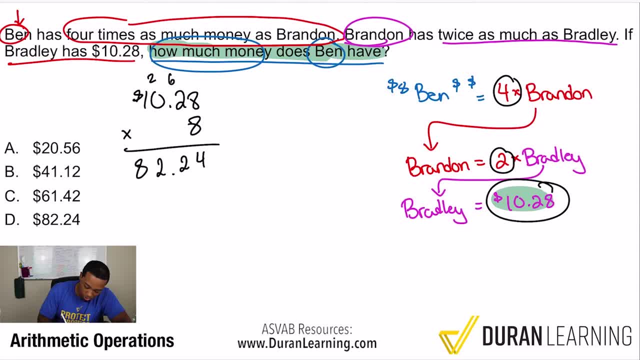 two there, And then you have the one times eight, which is eight, And so you have $82 and 24 cents. That's what we end up with And that represents our final answer, because we ended up setting ourselves up. We started with the given information to connect it to what we needed to figure out. 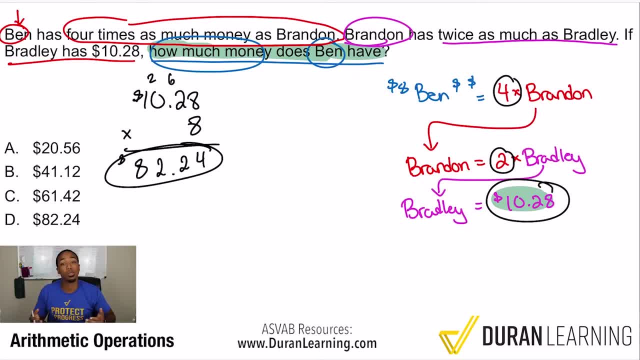 And once we had that set up, boom, then calculate, then go to town. The last thing you need to do is calculate, guys. the last thing, The first thing you need to do is just worry about the question itself, Because there's no point in looking at the numbers if you don't know what they represent. No, 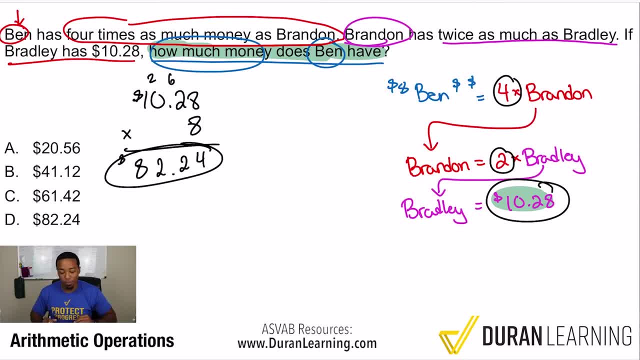 point at all, guys. no point at all. You have to start with the question: develop your plan, make sure your plan is good, and then go ahead and attack it with the calculations. And as you start this out for the first time, it's going to take a little while to really get it down to be. 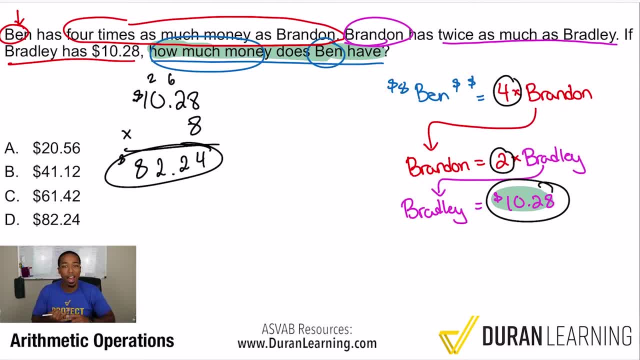 clear And only concern yourself with the question, because you're going to have decimals, you're going to have fractions, you're going to have percents. It's going to feel scary at first, but you have to discipline yourself to only focus on the question. The added bonus to this: the added 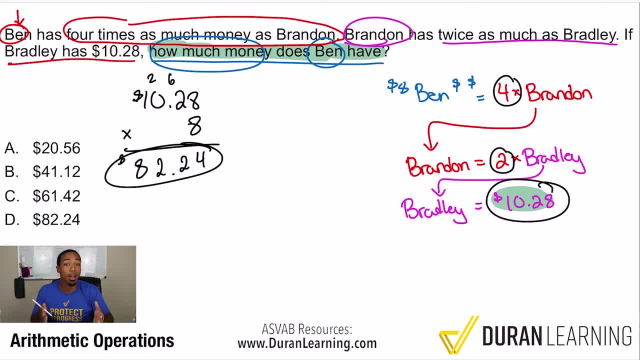 bonus to this is that you're going to be able to identify where you get stuck in the problem, Like if you're calculating and you don't know why you're calculating, boom, you're stuck right there because you are not understanding what the question is about. If you catch yourself not, 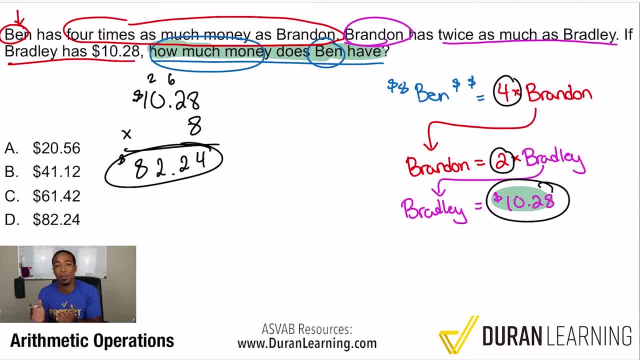 they represent no point at all, guys. no point at all. you have to start with the question: develop your plan, make sure your plan is good and then go ahead and attack it with the calculations. and as you start this out for the first time, it's going to take a little while to really get it down to be. 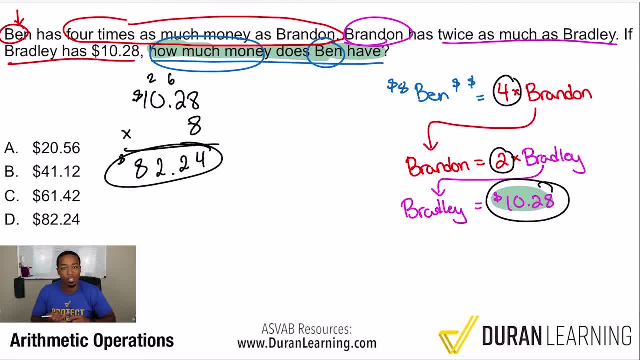 clear and then you're going to have to start with the question, because you're going to have decimals, you're going to have fractions, you're going to have percents. it's going to feel scary at first, but you have to discipline yourself to only focus on the question. the added bonus to 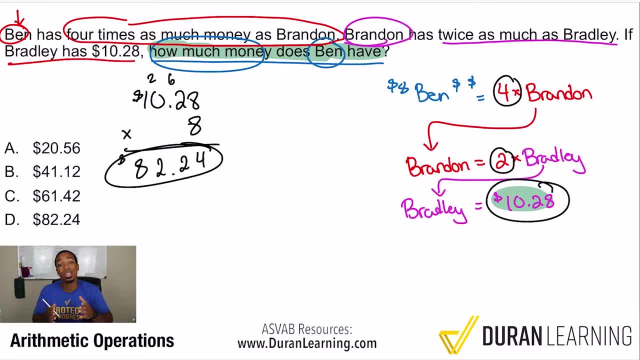 this. the added bonus to this is that you're going to be able to identify where you get stuck in the problem, like if you're calculating and you don't know why you're calculating, boom, you're stuck right there because you are not understanding what the question is about. if you catch yourself, 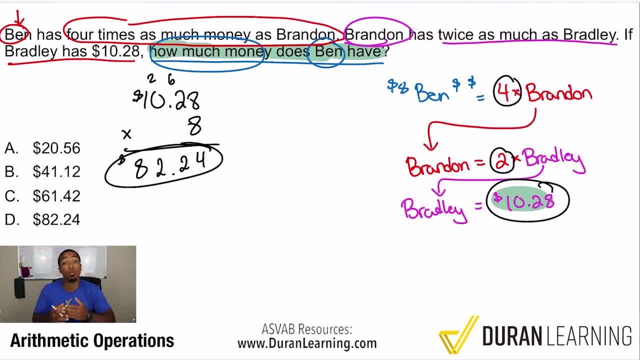 not being able to interpret what those key words are, then, boom, you need more practice just knowing what key words mean, and then you know like four times and twice you need to know what that means, and so if you catch yourself unable to make a plan, then it's really more so. 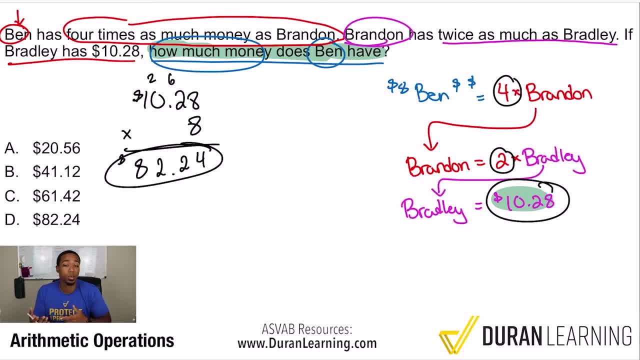 about your ability to translate the english into math. that's really what that's about. so you can check yourself at each three of these phases in terms of, again, what's the context like, what's the question then, what's the content like, what's the math that i need to use and the information that 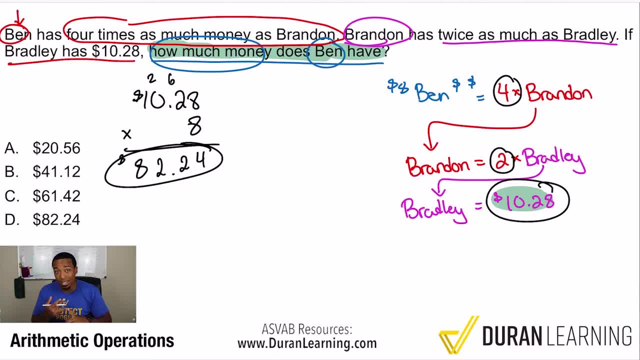 i'm solving the context, the story, then the content, the math, and then computation, which is calculating. and there it is. so let's go ahead and show ourselves question number two here and let's use this same strategy again: go straight to the question. so here we go straight to the question. 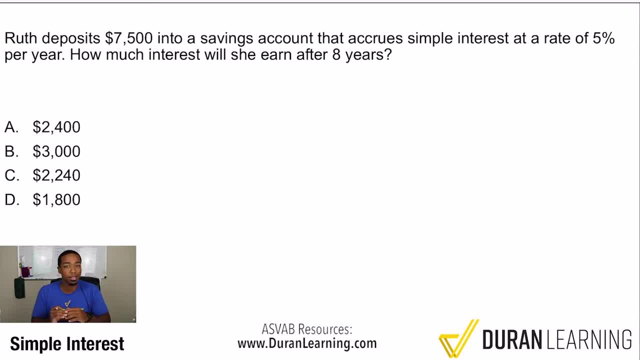 then go ahead and make that plan and then calculate at the end. so here we go. ruth deposits again. don't worry about that. we're going to go straight to the question: how much interest will she earn after eight years? all right, the key facts here, right there. 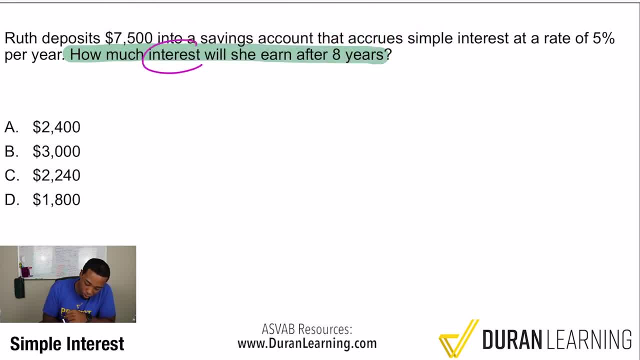 let me use purple actually to highlight this interest earned after eight years. right there, that's all you care about. those are the only keywords you care about interest, and after eight years now, when you read this question statement, you want to go ahead and ask yourself: well, what? 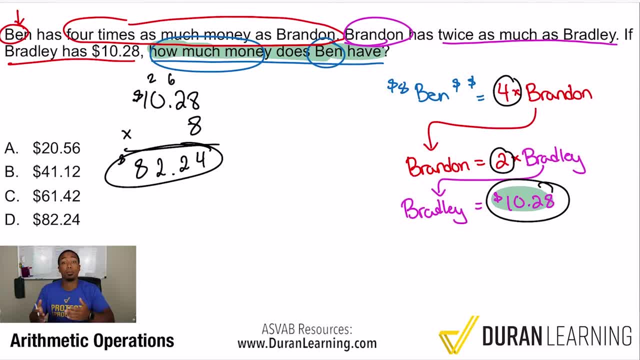 being able to interpret what those key words are, then, boom, you need more practice Just knowing what key words mean, And then you know, like four times and twice you need to know what that means, And so if you catch yourself unable to make a plan, then it's really more so. 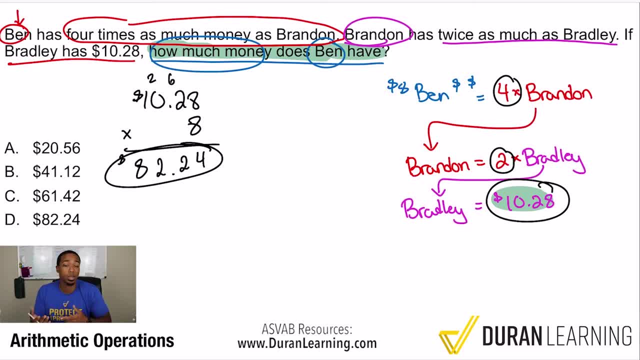 about your ability to translate the English into math. That's really what that's about. So you can check yourself at each three of these phases in terms of, again, what's the context Like, what's the question, Then what's the content Like, what's the math that I need to use and the information. 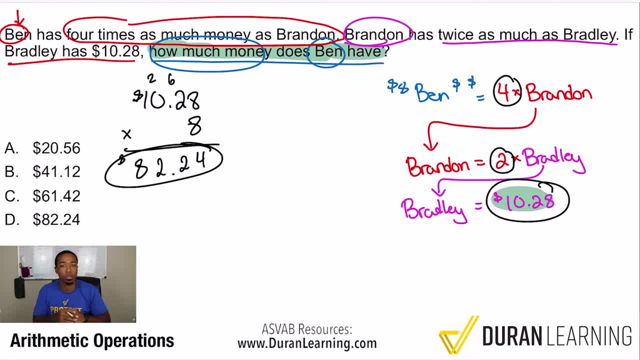 that I'm using, And then the calculation. These are the three Cs to problem solving: The context, the story, then the content, the math, and then computation, which is calculating. And there it is. So let's go ahead and show ourselves. question number two: 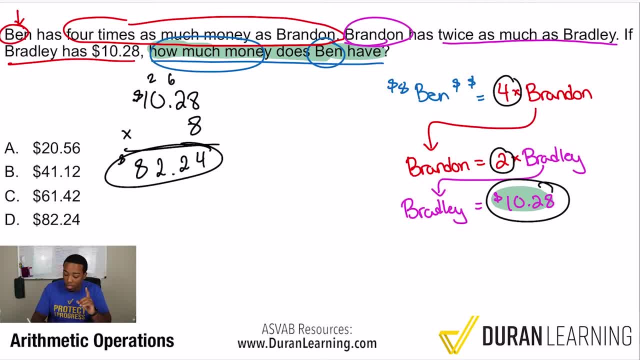 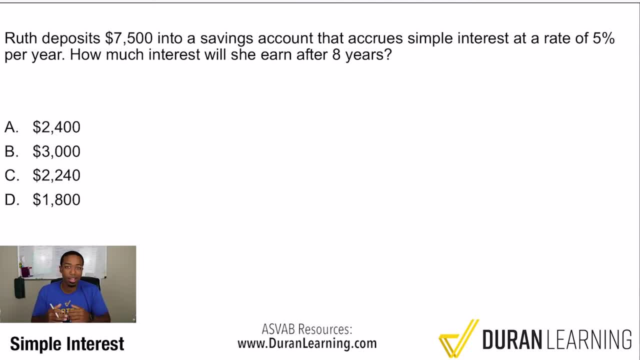 here And let's use this same strategy Again: go straight to the question. So here we go straight to the question. then go ahead and make that plan and then calculate at the end. So here we go. Ruth deposits- Again, don't worry about that, We're going to go straight to. 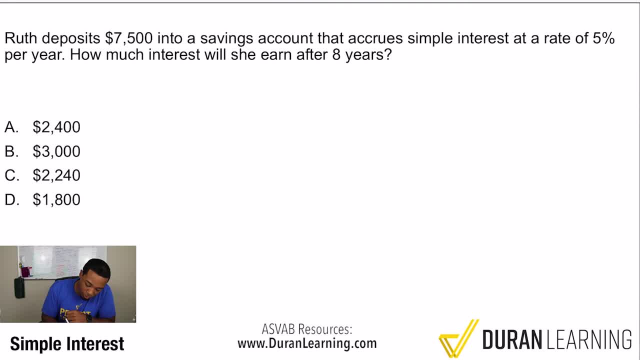 the question: How much interest will she earn after eight years? All right, The key facts here, right there. Let me use purple actually to highlight this: Interest earned after eight years. Right there, That's all you care about. Those are the only keywords. you care about Interest. 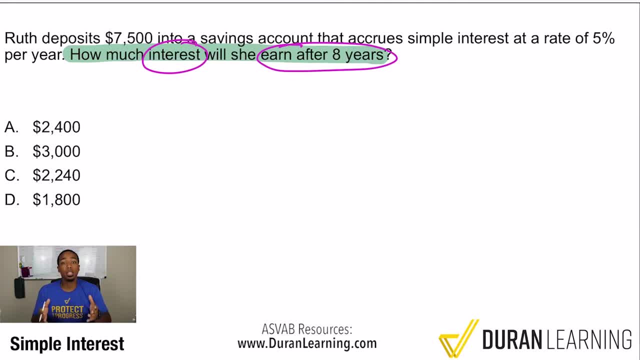 and after eight years. Now, when you read this question statement, you want to go ahead and ask yourself: well, what is it that I know about interest? And after eight years, that just seems like it's a condition of the problem. They're just saying. 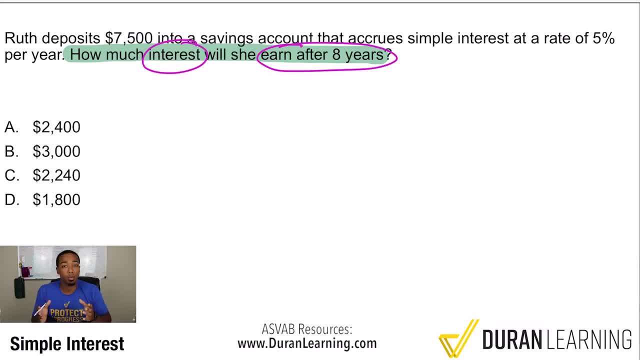 hey, after this amount of time. But what do you know about interest? Well, remember there are two types of interest here on the ASVAB: One is simple interest and the other is compound interest. So just to be very clear, you should be fishing in your mind for this information. 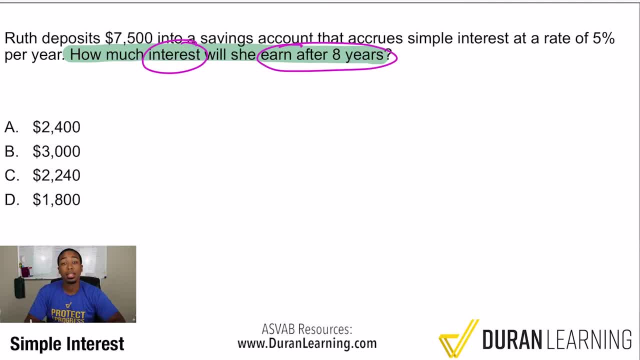 before you actually go into the actual word problem. This is because you want to warm yourself up. You need to be ready to use the information that you have in any formula or any procedure or any equation. You need to be ready to use the information that you have in any formula or any. 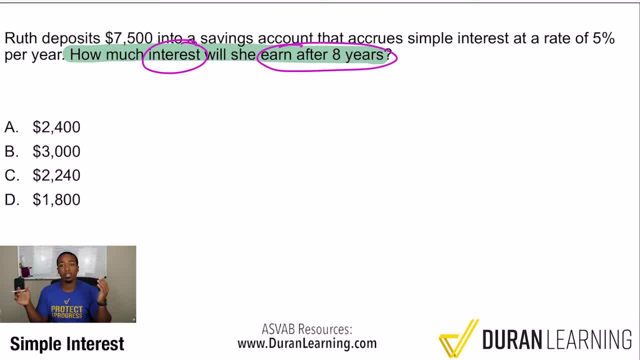 is it that i know about interest and And after eight years that just seems like it's a condition of the problem. They're just saying hey after this amount of time, But what do you know about interest? Well, remember there are two types of interest here. on the ASVAB. 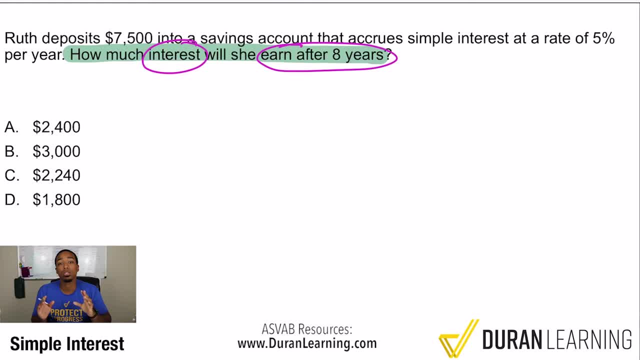 One is simple interest and the other is compound interest. So, just to be very clear, you should be fishing in your mind for this information before you actually go into the actual word problem. This is because you want to warm yourself up. You need to be ready to use the information that you have in any formula or any procedure. 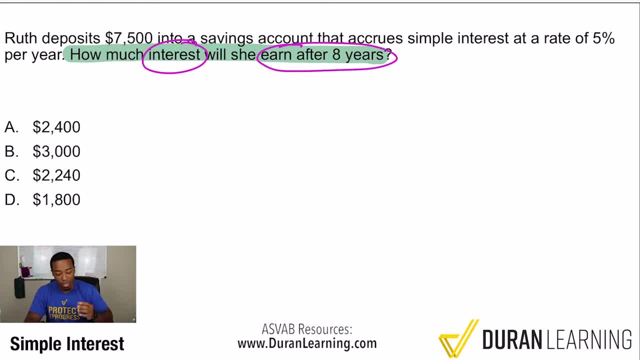 or any equation that it's useful in. So again, interest, simple and compound. Simple interest is simply put: you just go ahead and find the interest one time and you keep earning that amount every year, or however long they're saying. But again, simple interest. you only calculate the interest once and then you just multiply it. 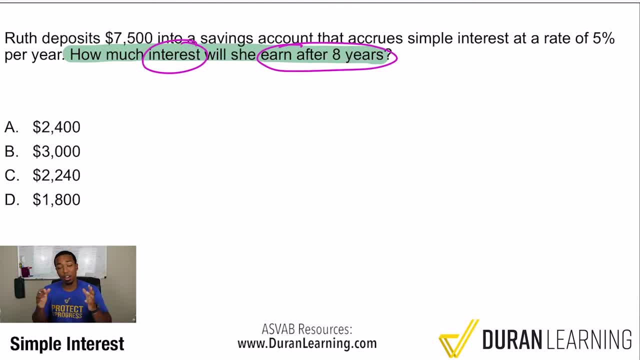 Now, with compound interest, it's like this: If I have $100 in the bank and I earn my interest, and now I have $105 in the bank, I earn interest on the $105.. And then boom, let's say next year it's like $112, then I'll earn interest on that. 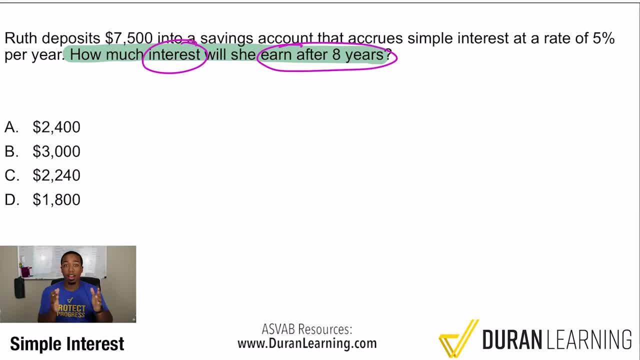 With simple interest. if I put in $100, I'm only ever earning interest on the $100, not what I earned because of it. It's not compounding, It's just simple interest. You keep it simple. So if that didn't make too much sense, no worries. 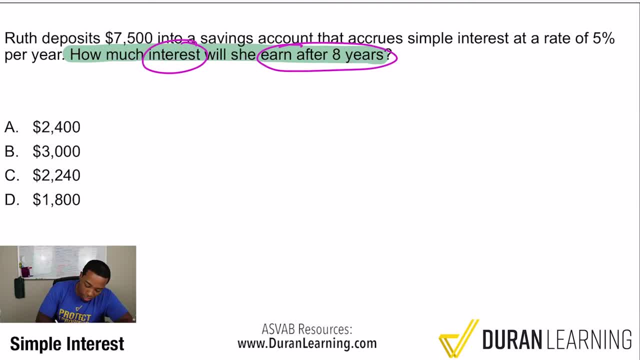 Let's get to it. So again we're worried about interest. After eight years I know that there's two types of interest And I clearly see right here occurs simple interest. So in your mind, you need to be ready, You need to be ready. 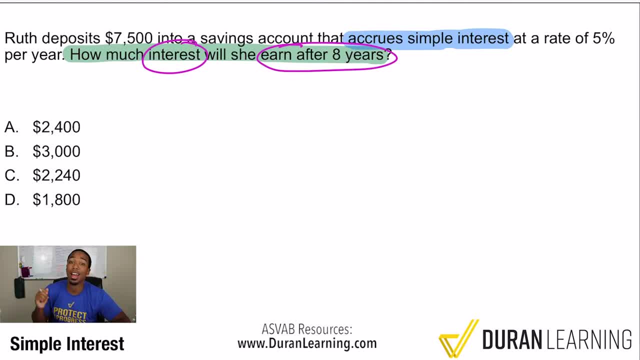 You need to be ready. You need to be locked and loaded and ready to go thinking that, boom, simple interest. I know exactly what that means. It means that I'm only going to use the principal amount or the starting amount and consider interest from there. 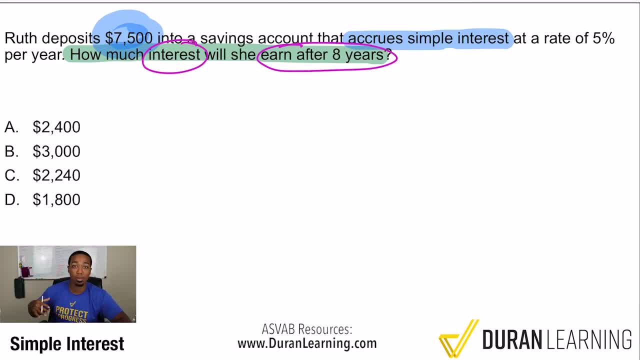 The interest that I earn is not going to count back to what I'm taking the interest of. Again, it's only the $7,500 there. So again, root deposits that much money into the savings account, that occurs the interest. 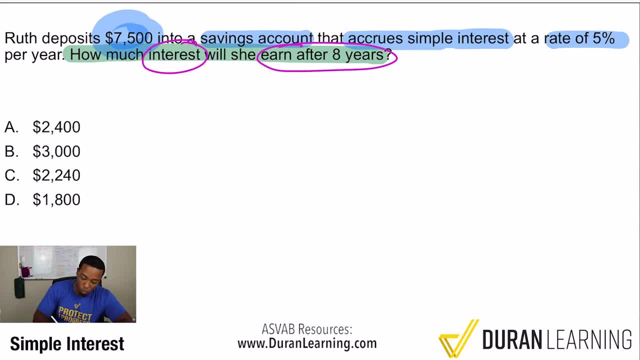 The rate is 5% per year. So, with that said, because it's simple, simple interest, we're going to go ahead and set it up the following way: We're going to say that we are looking for 5% of $7,500. 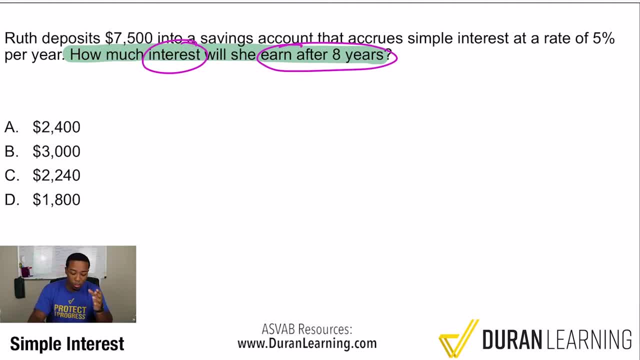 equation that it's useful in. So again, interest simple and compound. Simple interest is simply put: You just go ahead and find the interest one time and you keep earning that amount every year, or however long they're saying. But again, simple interest. you only calculate the interest once and 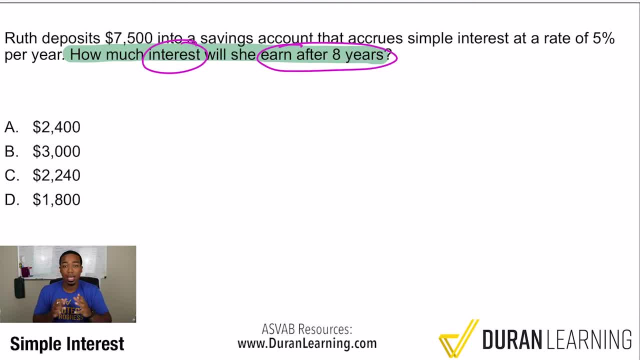 then you just multiply it. Now, with compound interest it's like this: If I have $100 in the bank and I earn my interest, and now I have $105 in the bank, I earn interest on the $105. And then 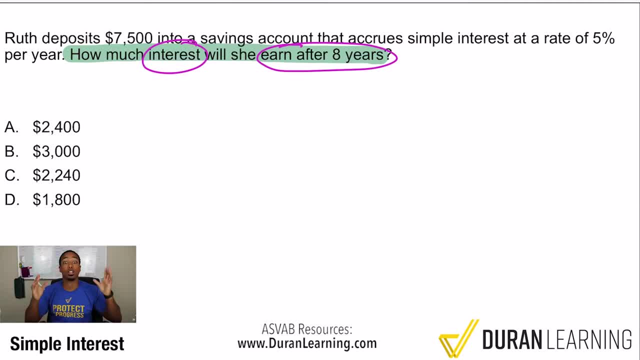 let's say next year it's like $112, then I'll earn interest on that With simple interest. if I put in $100, I'm only ever earning interest on the $100, not what I earned because of it. It's. 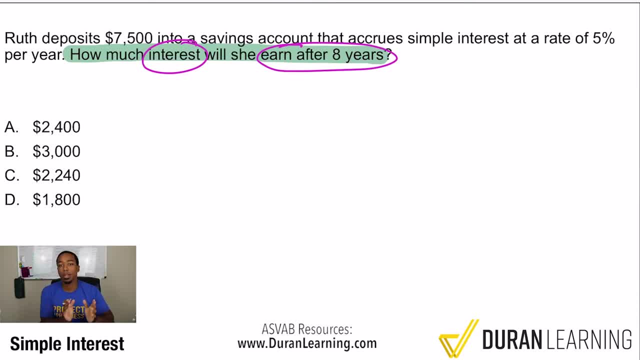 not compounding, It's just simple interest. You keep it simple. So if that didn't make too much sense, no worries, Let's get to it. So again we're worried about interest. After eight years I know that there's two types of interest And I clearly see right here occurs simple interest. 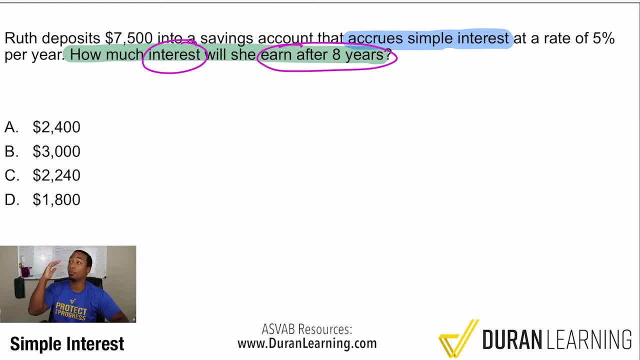 So in your mind you need to be locked and loaded and ready to go, Thinking that boom, simple interest. I know exactly what that means. It means that I'm only going to use the principal amount or the starting amount and consider interest from there. The 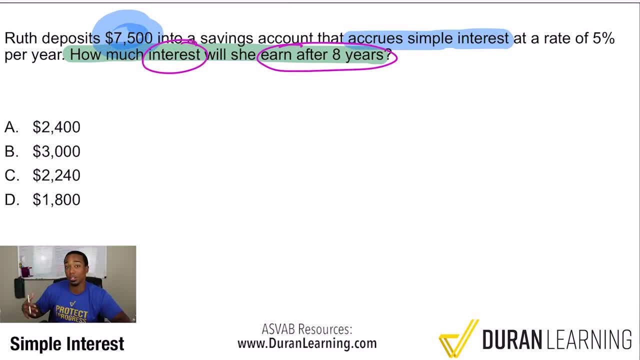 interest that I earn is not going to count back to what I'm taking the interest of. Again, it's only the $7,500 there. So again, root deposits that much money into the savings account. that occurs the interest the rate is 5% per year. So with that said, because it's simple interest, 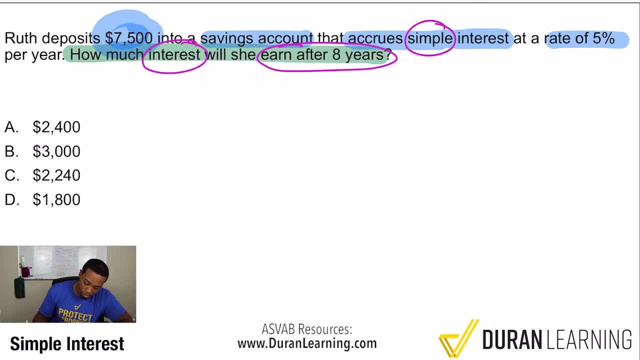 we're going to use the principal amount or the starting amount and consider interest from there. We're going to go ahead and set it up the following way: We're going to say that we are looking for 5% of $7,500. And that's going to give us one year of interest Because we're looking 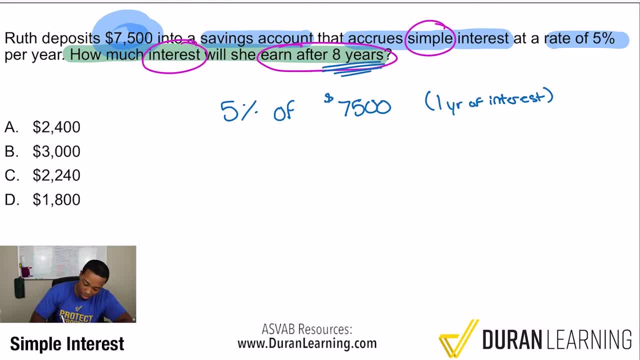 for eight years. we will then take this and then multiply by eight, Multiply by eight years. So does that make sense? So we're going to go ahead and set it up the following way: We're going to say that we are looking for 5% of $7,500. And that's going to give us one year of interest, Because we're going 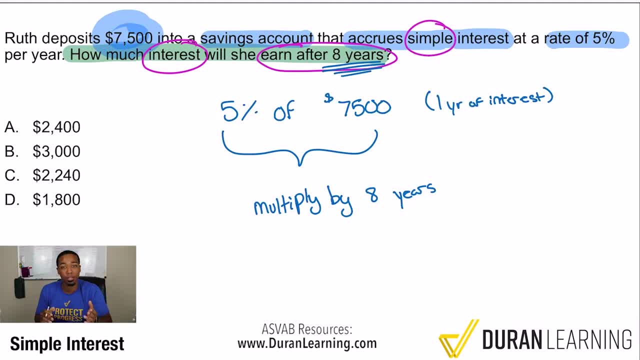 to say that we are looking for 5% of $7,500. And that's going to give us one year of interest. Does it truly make sense? Because if it doesn't pause the video, go back a couple of seconds here. 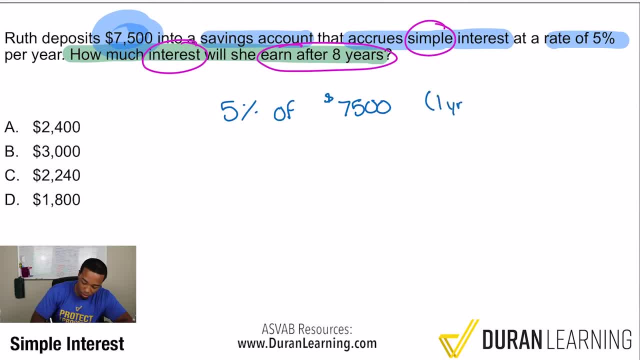 All right, And that's going to give us one year of interest, Because we're looking for eight years. we will then take this and then multiply by eight. Whoops, Multiply by eight years. So does that make sense? Does it truly make sense? 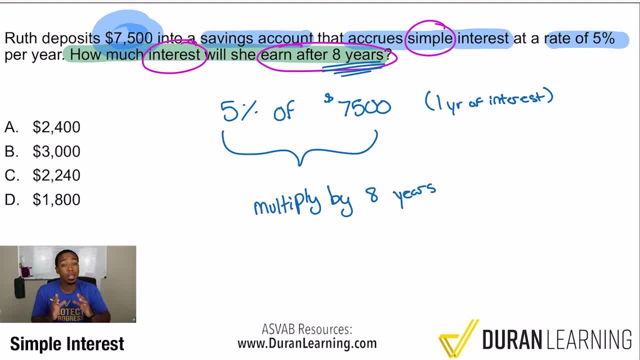 Because if it doesn't pause the video, go back a couple of seconds here and really hear me out in explaining it again, Because it's way too important for you to miss this right now. Again, I started off with the question: interest after eight years. 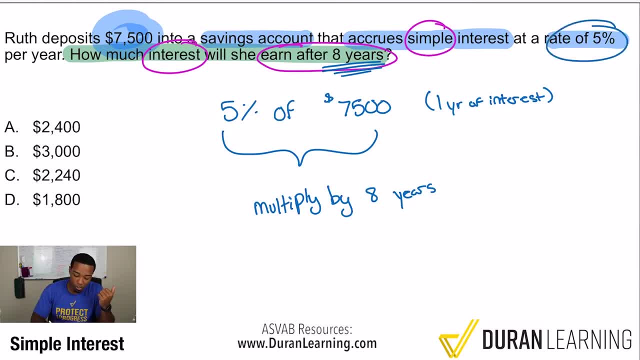 I just looked for wherever interest was stated- 5% interest- And I know I need a deposit or an initial amount or starting amount, which is right there. And what type of interest is it though? Oh, simple interest. So boom, as long as you know your basic sets of facts about interest. 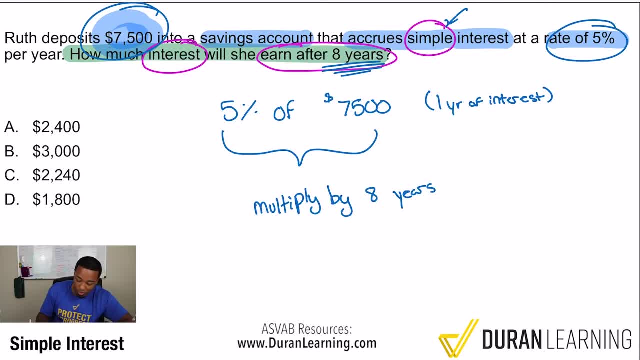 the rest is gravy. It really is, Because now all I have to do is take 5% of $7,500.. Step one, Step two, multiply by eight years, My plan is done. Now we just have to quickly calculate and that's it. 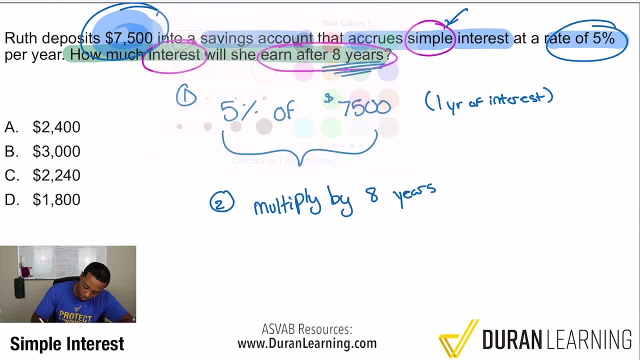 So, first up, number one: what I'll do is I'll go ahead and take that 5% of $7,500.. How do you do that? again, Remember, before you multiply percents and numbers, you need to go ahead and convert that percent to a decimal. 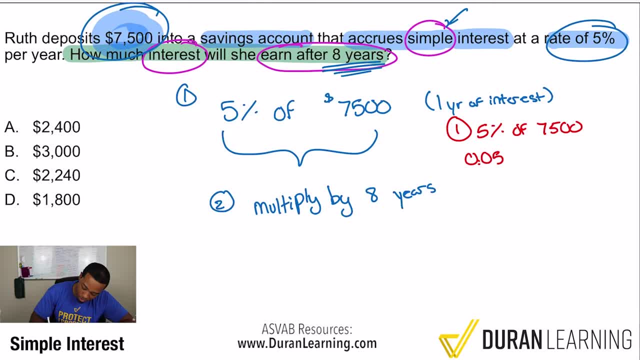 So, with that said, this is 0.05.. Multiply by 7,500.. Remember percent per cent per 100 or out of 100. So to turn 5% into a decimal divided by 100, which moves the decimal place over to the left two times. 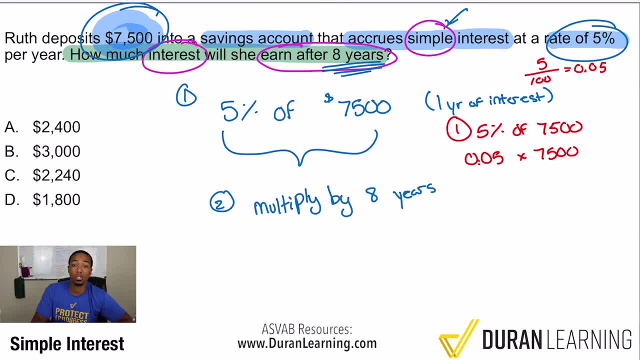 So 0.05,, not 0.005,, not 0.5, just 0.05.. So, with that said, let's go ahead and do that calculation And what we're going to get is well, whatever we're going to get. 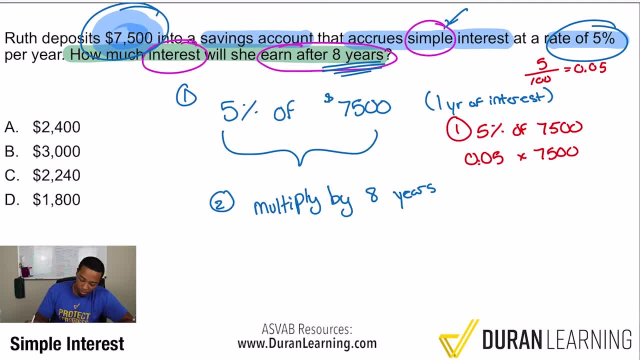 But let me go ahead. I'm going to throw some mental math your way to help you out, Because, whatever this is, you want to multiply it by eight. So, technically speaking, again this is being multiplied by eight. So, technically speaking, you're multiplying by eight after the fact. 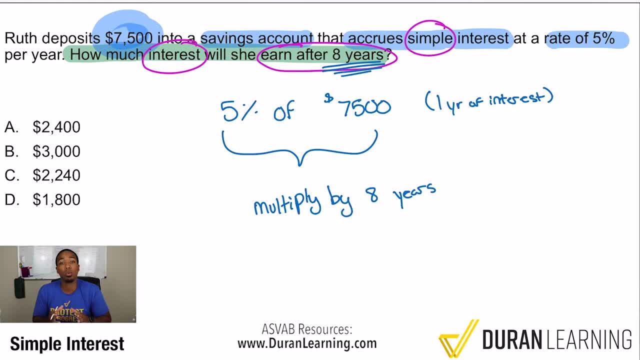 and really hear me out in explaining it again, Because it's way too important for you to miss this right now Again. I started off with the question interest. after eight years, I just looked for wherever interest was stated 5% interest, And I know I need a deposit or an initial. 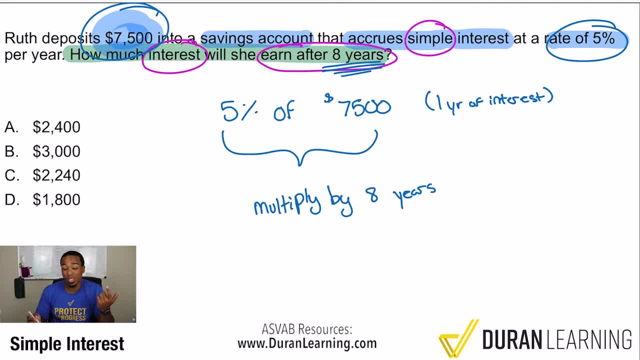 amount, or starting amount, which was right there. And what type of interest is it, though? Oh, simple interest, So boom. as long as you know your basic sets of facts about interest, the rest is gravy. It really is, Because now all I have to do is take 5% of $7,500.. Step one, Step two: multiply by. 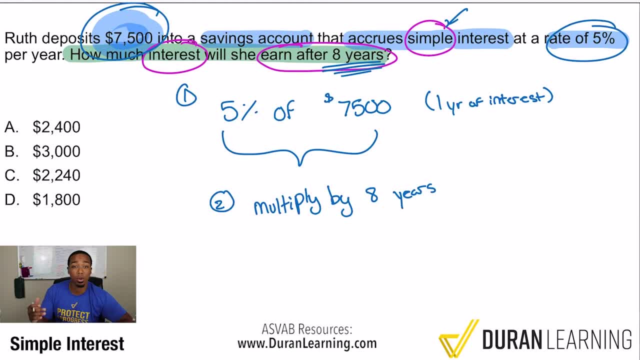 eight years. My plan is done. Now I just have to quickly calculate and that's it. So first step, number one, what I'll do is I'll go ahead and take that 5% of $7,500.. How do you do that again? 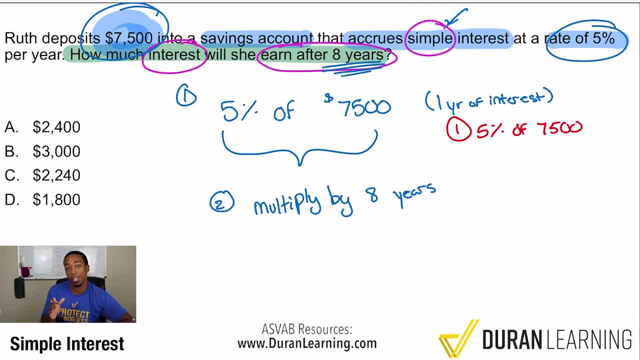 Remember, before you multiply percents and numbers, you need to go ahead and convert that percent to a decimal. So, with that said, this is 0.05, multiply by 7,500.. Remember percent per cent per 100 or out of 100. So to turn 5% into a decimal. 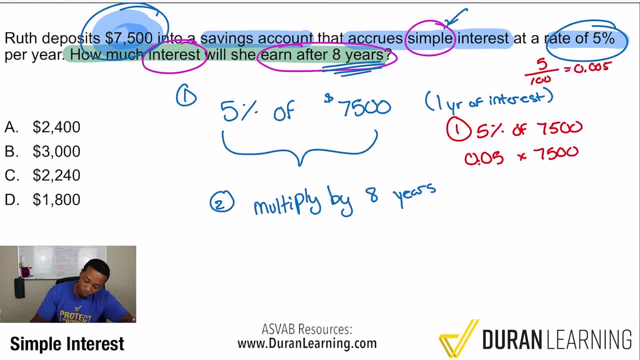 divided by 100, which moves the decimal place over to the left two times, So 0.05, not 0.005, not 0.5, just 0.05.. So, with that said, let's go ahead and do that calculation. 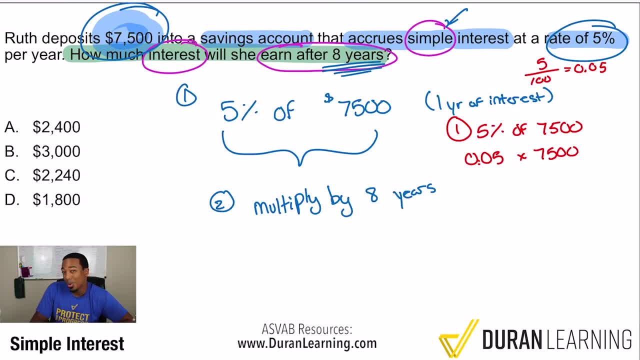 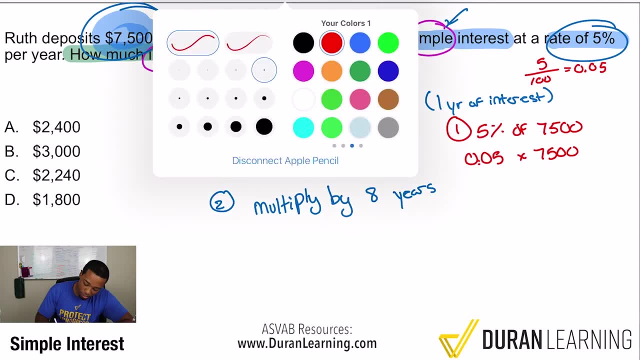 And what we're going to get is well, whatever we're going to get, But let me go ahead and throw some mental math your way to help you out, Because whatever this is, you want to multiply it by eight. So, technically speaking, again this is being multiplied by eight. 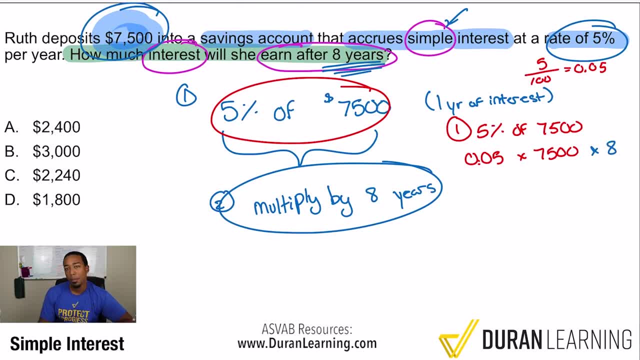 So, technically speaking, you're multiplying by eight after the fact- But remember this, everybody, because again, I'm always trying to save you time- Why multiply by 0.05 and then multiply by eight? Why not just kind of help yourself out? And here's what I mean: 0.05 times. 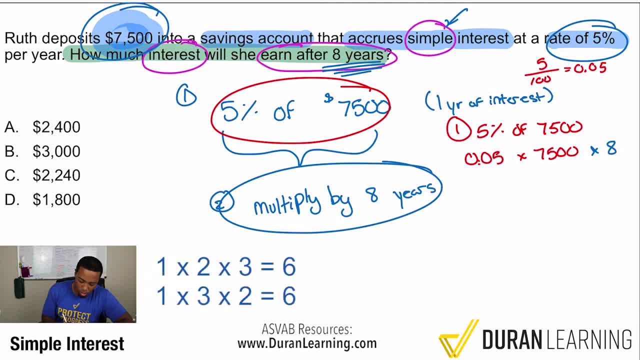 7,500 times eight. Think about it like this: Is 1.05 times 7,500 times eight. Is 1.05 times 7,500 times one times two times three, the same as one times three times two. The answer is yes, They're both. 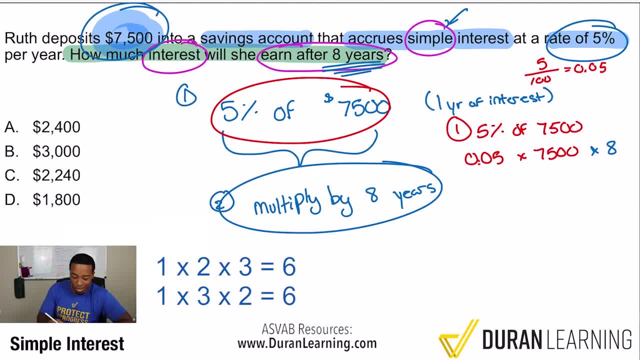 six. They're both going to end up being six, And so really, what I'm trying to get at here is that you can actually shift this over and just say 0.05 times eight times 7,500.. That's going to make my 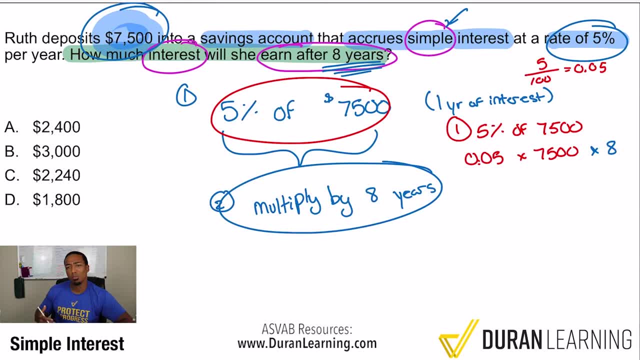 But remember this everybody, because again, I'm always trying to save you time: Why multiply by 0.05 and then multiply by eight? Why not just kind of help yourself out? And here's what I mean: 0.05 times 7,500 times eight. 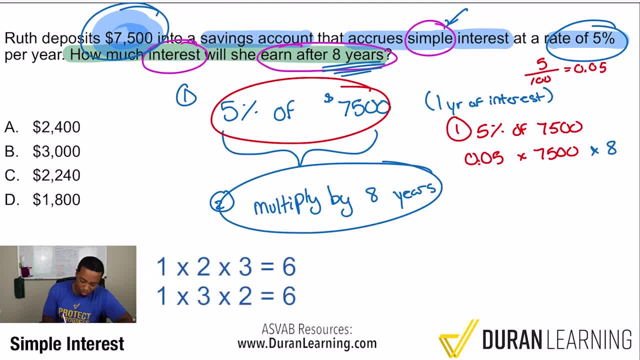 Think about it like this: 1 times 2 times 3, the same as 1 times 3 times 2.. The answer is yes, They're both six, They're both going to end up being six, And so, really, what I'm trying to get at here is that you can actually shift this over and just say 0.05 times 8 times 7,500. 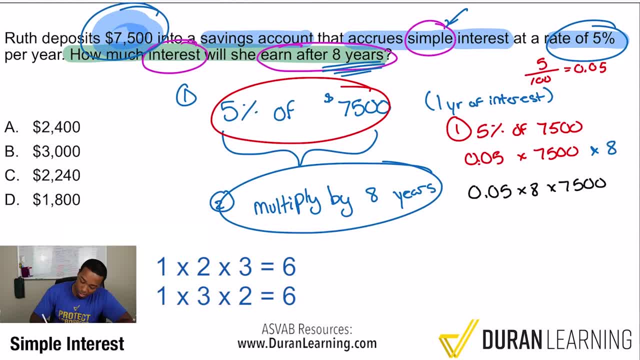 That's going to make my life a lot easier. You want to know why? It's because 0.05 times 8 gives you 0.4 or 0.40, whichever way you want to say it. You can multiply it like this: 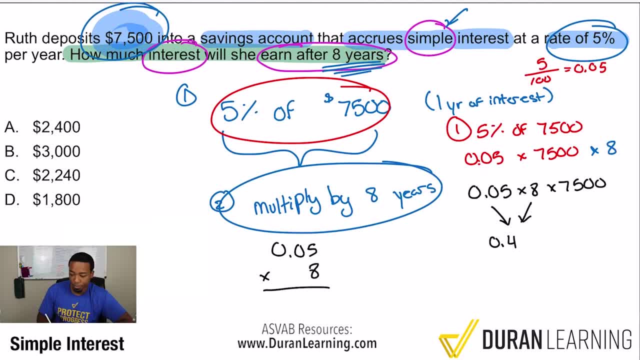 0.05 times 8 gives you 0.4 or 0.40, whichever way you want to say it. You can multiply it like this, You multiply it like that, And when you do it, just make sure that you're putting the decimal place back in its place. 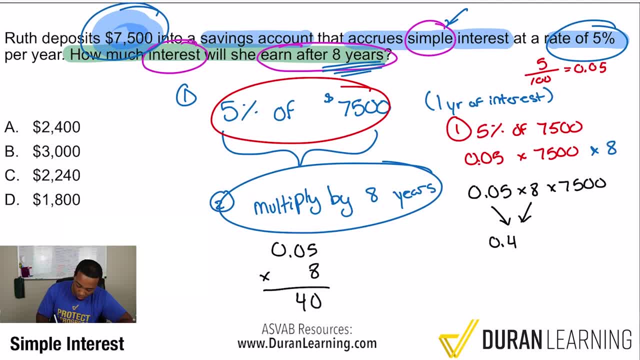 So 5 times 8, that gives you 40. And since you had two decimal places, go ahead and put that back. So again, that gives you 0.40 or 0.4, whichever way you want to consider it. 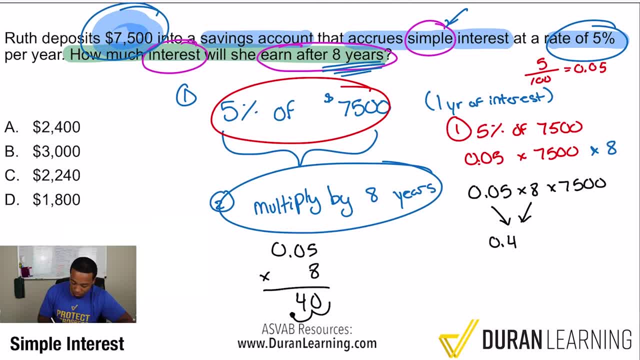 So with that said from there, what we're going to do is take that 0.4 and we're going to multiply it by that 7,500.. So, with that said, that's going to be pretty easy right there. So just move the decimal place back one time once you have it. 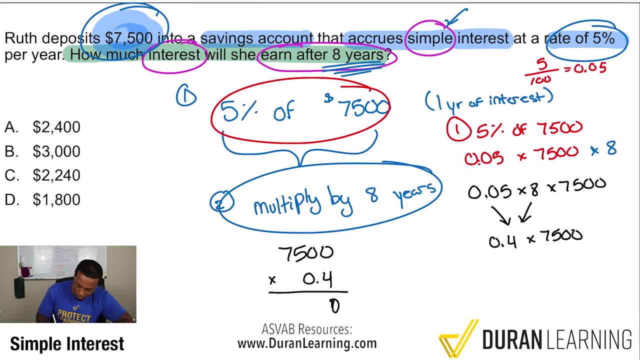 And here we go: 0 times 4, that's 0.. 0 times 4, again 0.. 5 times 4, that's 20.. Put that there And then 7 times 4 is 28 plus 2 is 30.. 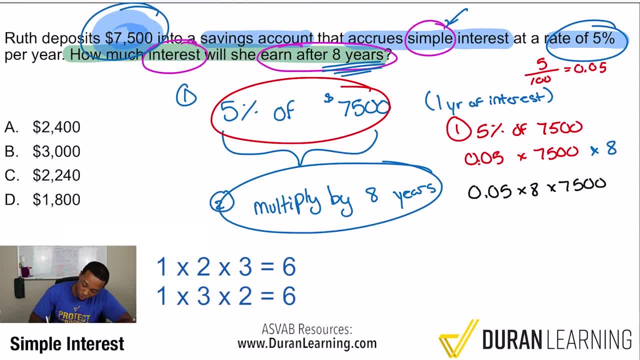 life a lot easier. You want to know why? It's because 0.05 times eight gives you 0.4 or 0.40, whichever way you want to say it. You can multiply it like that, And when you do it, just make sure that you're putting the decimal place back in its place. So 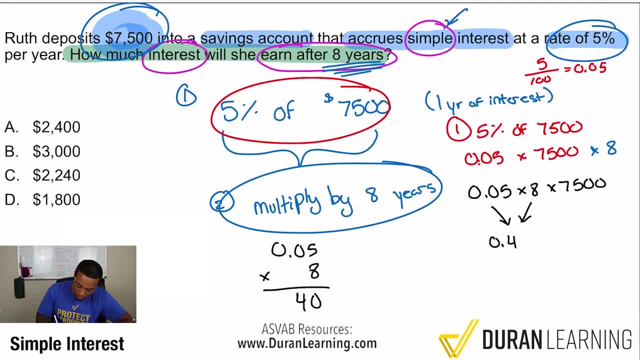 five times eight, that gives you 40. And since you had two decimal places, go ahead and put that back. So again, that gives you 0.40 or 0.4, whichever way you want to consider it. So with 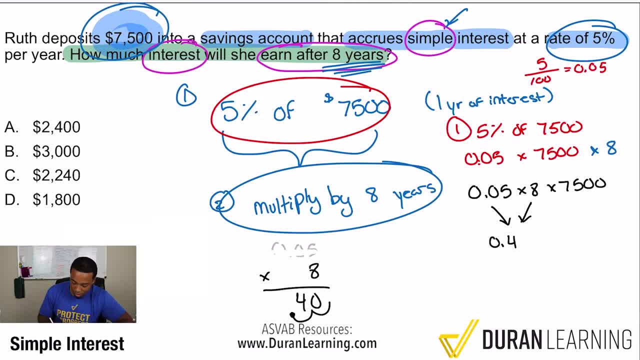 that said. from there, what we're going to do is take that 0.4 and we're going to multiply it by that 7,500.. So, with that said, that's going to be pretty easy, right there. So just move the decimal place back one time once you have it, And here we go. 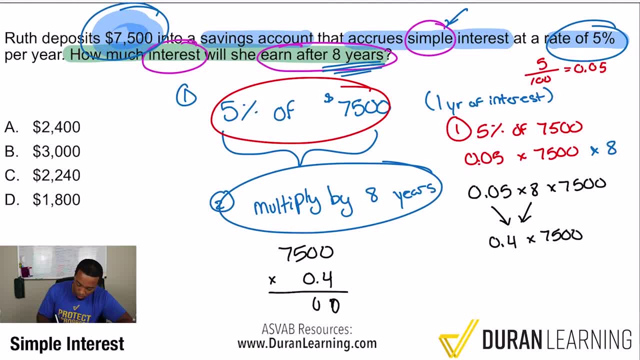 Zero times four, that's zero. Zero times four, again zero. Five times four, that's 20.. Put that there. And then, seven times four is 28 plus two is 30. Take that decimal place and put it back. 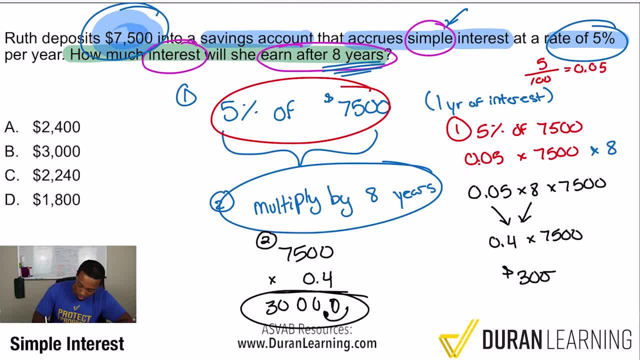 So that's going to give us 3,000.. And there we go. That's how much you'll earn after eight years. Specifically, that's how much Ruth will earn after eight years. But again, guys, it's not about the. 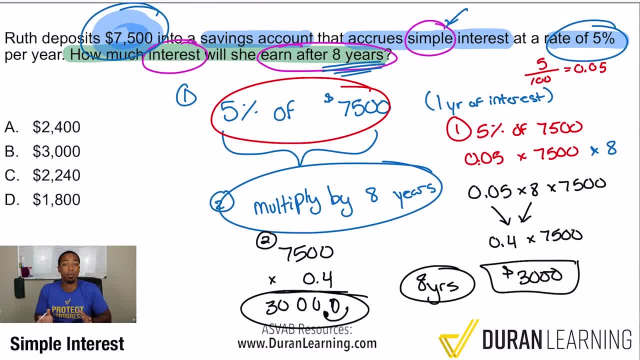 calculations. That's the last step. Those are the last steps to every problem. The first steps are always going to be again. what's my question? Keywords Connect it back to the problem. And there we go: Make your plan and follow it. The more you can do that. 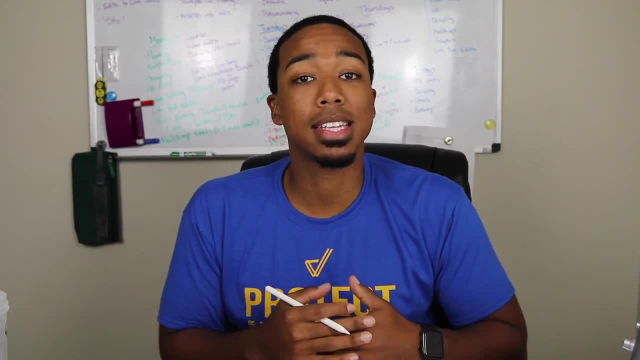 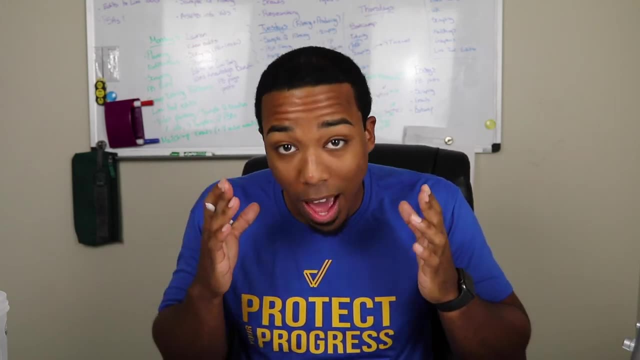 the better you'll end up. I can promise you that right now. This is not going to happen by luck. This is not going to happen by hoping and wishing when you see those numbers and just try to add them together or subtract them or whatever. You have to- absolutely have to- have a game plan when you start every. 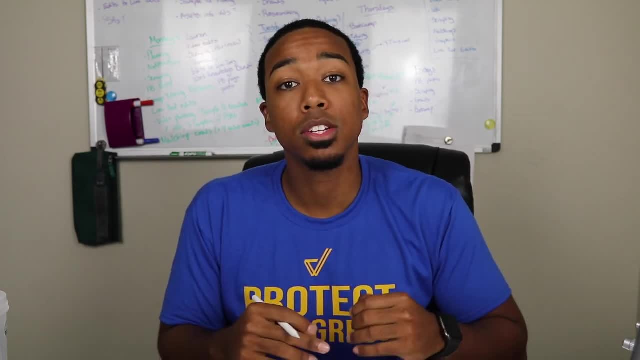 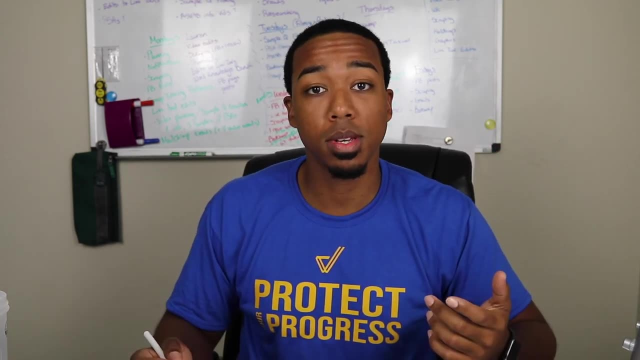 single problem. And so, again, it's the three C's of problem solving. Start off with the context, the story, the problem itself, like the question, Highlight those keywords. What do those keywords mean? Okay, cool, I remember what they mean. Now let's go back into the problem. Let's go for that. 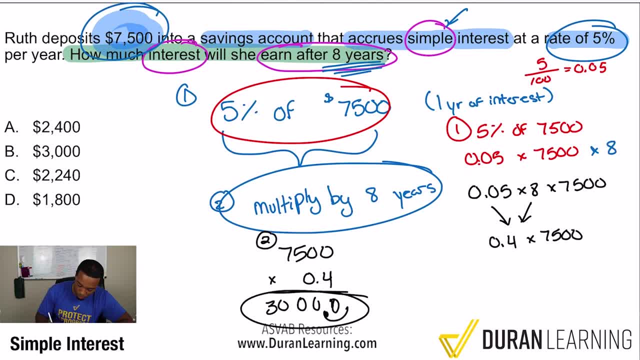 Take that decimal place and put it back. We're going to multiply that by 0.4.. So it's now 8 times 4, that gives us 30.. And there we go. That's how much you'll earn after eight years. 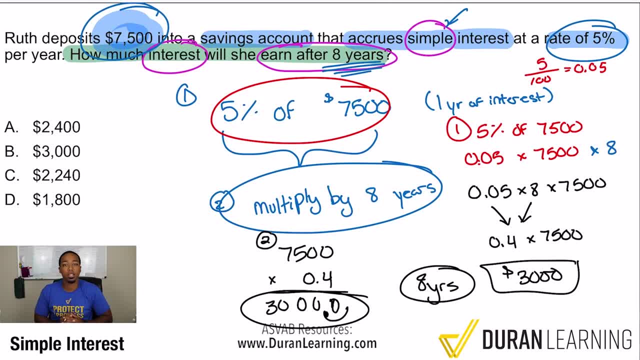 Specifically, that's how much Ruth will earn after eight years. But again, guys, it's not about the calculations. That's the last step. Those are the last steps to every problem. The first steps are always going to be again. what's my question? 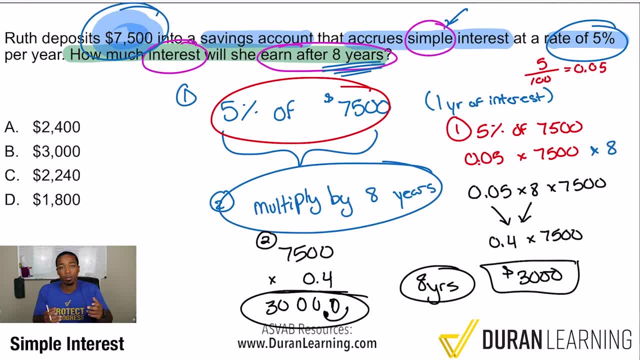 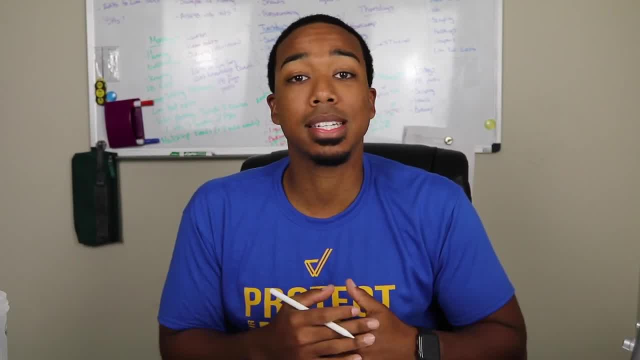 Keywords Connect it back to the problem. And there we go: Make your plan and follow it. The more you can do that, the better you'll end up being. I can promise you that right now, This is not going to happen by luck. This is 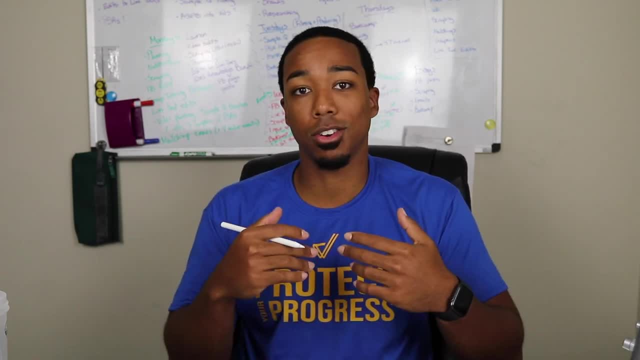 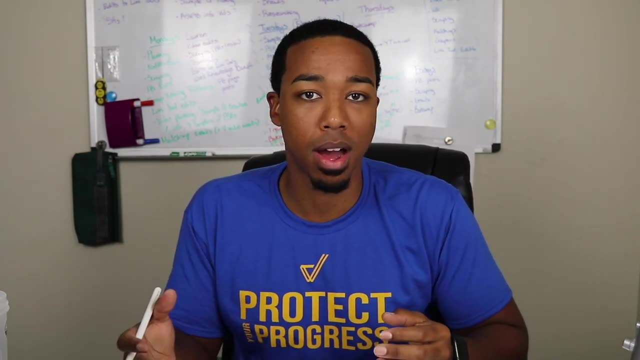 not going to happen by hoping and wishing. when you see those numbers and just try to add them together or subtract them or whatever. You have to, absolutely have to have a game plan when you start every single problem. And so again, it's the three C's of problem solving. Start off with the 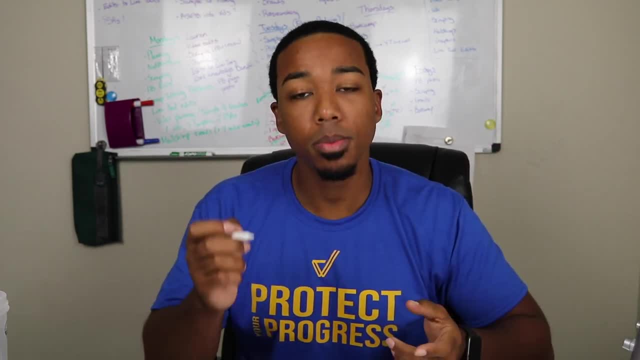 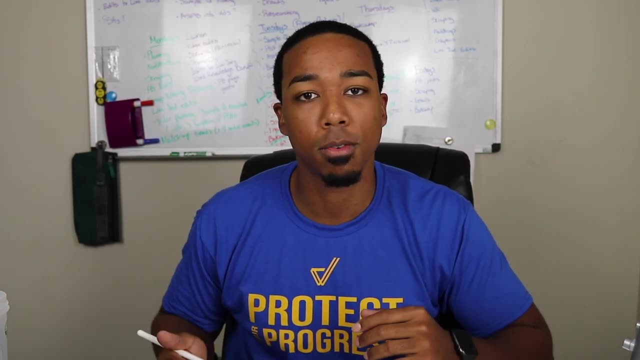 context, the story, the problem itself, like the question, Highlight those keywords. What do those keywords mean? Okay, cool, I remember what they mean. Now let's go back into the problem. Let's go for that information that we need, set it all up And then, once we have our setup right, once we 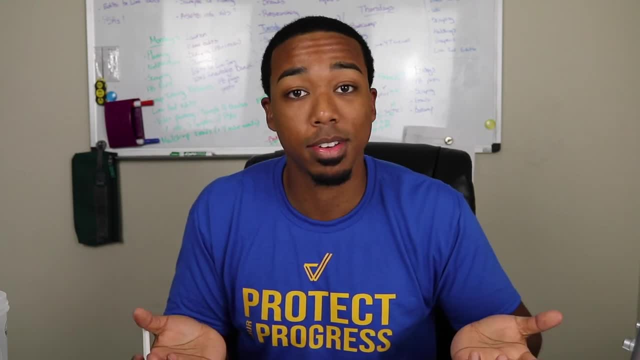 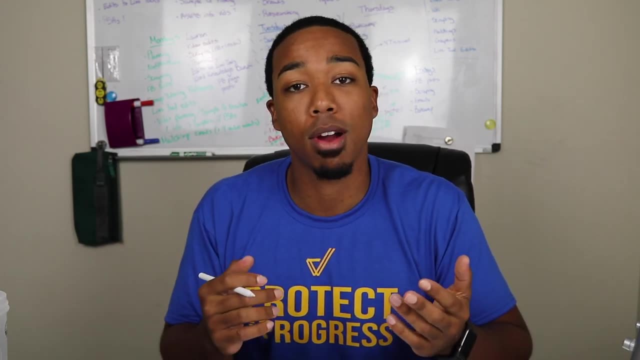 have the blueprint to the building. remember: you don't want to build a building without a blueprint because obviously people are going to die. So you want to go ahead, plan that thing out and then be absolutely sure that you're going to execute it the proper way. That's how your confidence can. 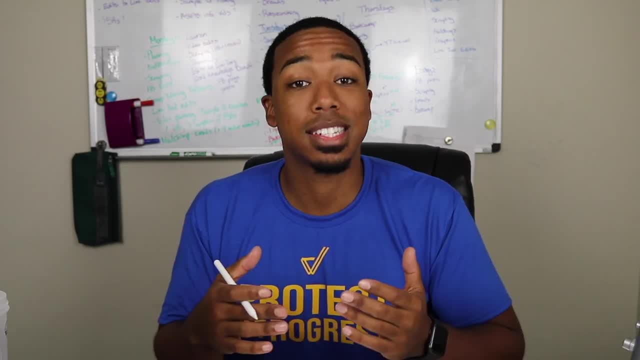 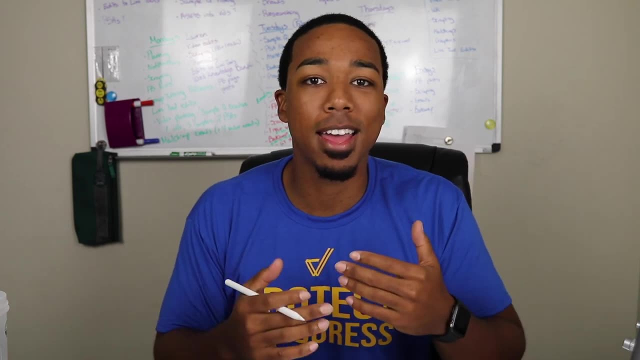 skyrocket. That's how your chances of being correct skyrocket. That's how you can finish one problem and know that you'll get the next one right. But if you're not employing any sort of strategy when you're doing work, you're not going to be able to do it. So if you're not employing any sort of 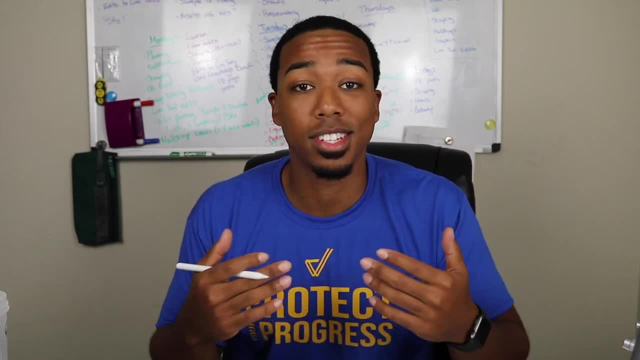 strategy, you're not going to be able to do it. So if you're not employing any sort of strategy when you're, then every work problem is going to feel like a brand new one every single time. But I promise you there's a connection between all of them. So again, guys, I'm Anderson, your ASVAB coach. 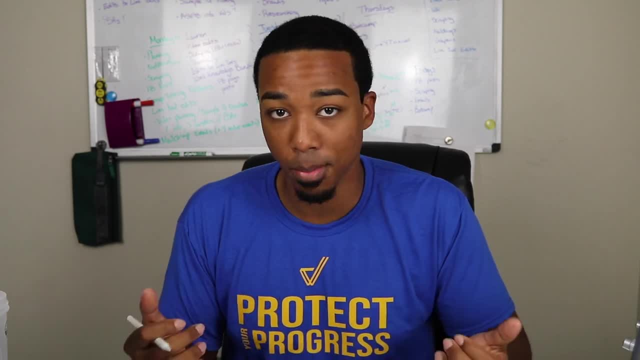 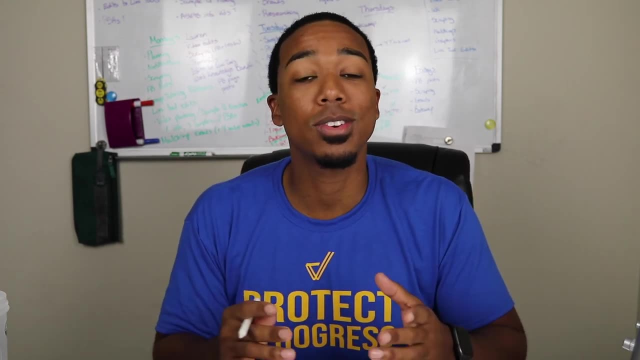 I hope you learned today how to tackle work problems the right way with me, And if you have any questions, just go ahead and comment on this video And if you liked it, give it a like, But don't forget to subscribe to this channel, That way you can get more videos just like this. So 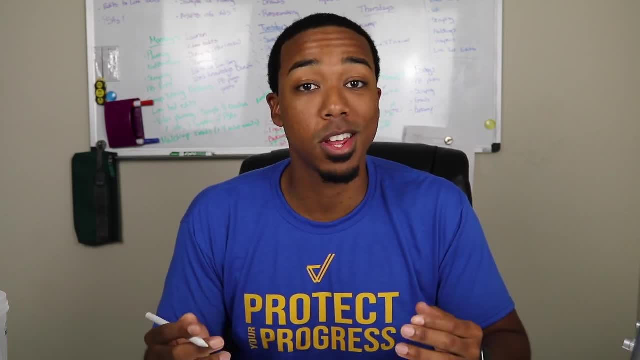 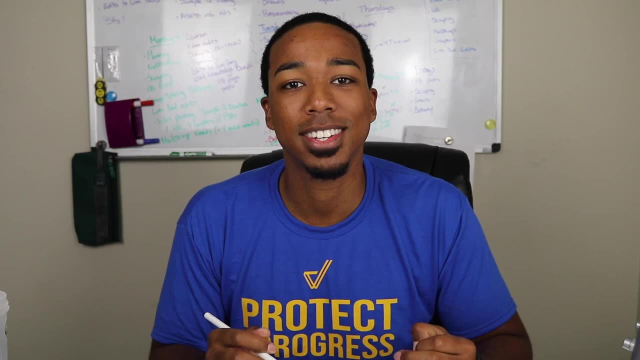 with. that said, everybody, if you have any questions, you can always reach out to me. Check the description of this video for all of our free and paid ASVAB resources to help you pass on your next attempt. Again, I'm Anderson, your ASVAB coach, and I'll see you in the next video.